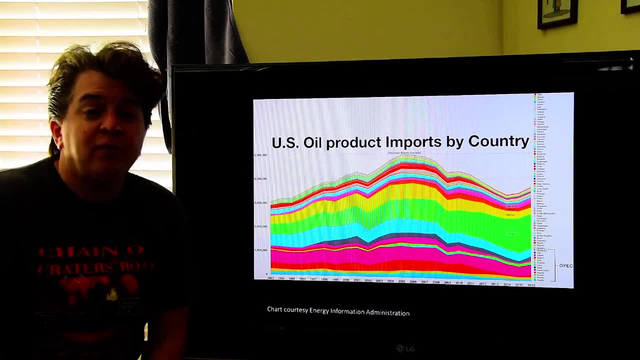 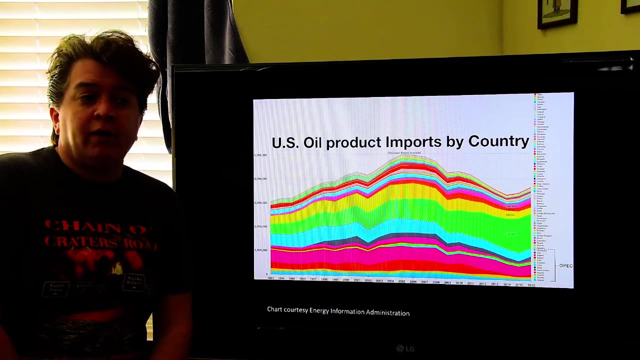 Today's topic is going to be energy resources. We're going to start off with conventional energy resources, like fossil fuels, and then take a look at some of the alternative energy resources. And I decided since, of course, we live in oil country here, right outside. 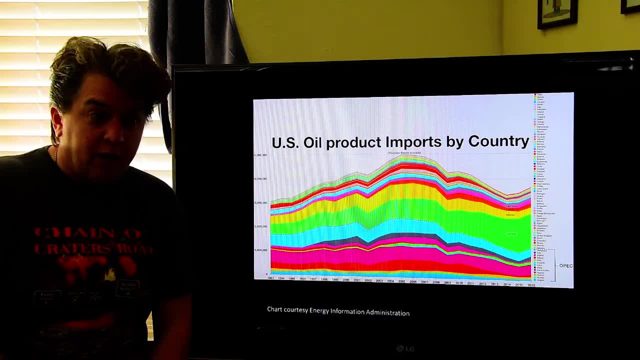 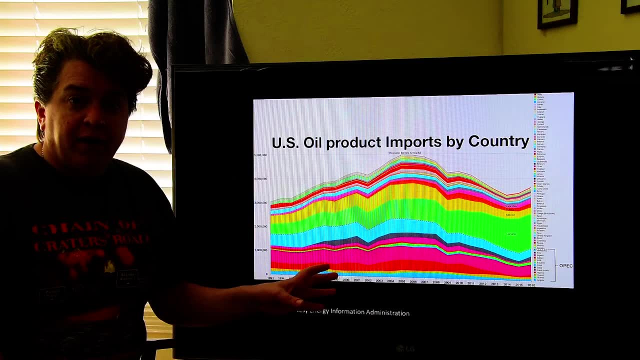 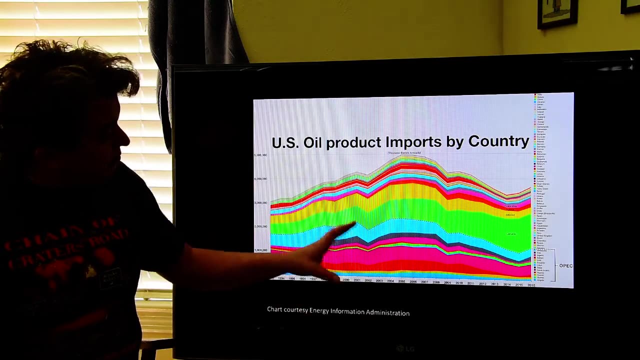 of Houston, I decided to start with crude oil as an energy source, And what I'm showing here, this is a graph showing imports to the US by country. Now, mind you, the US does produce quite a bit of its own oil domestically, But when it comes to imports, underneath this, 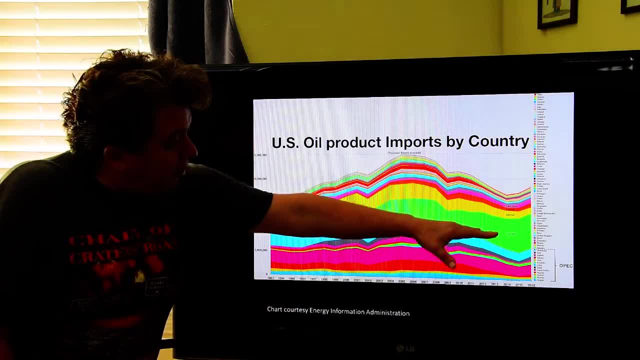 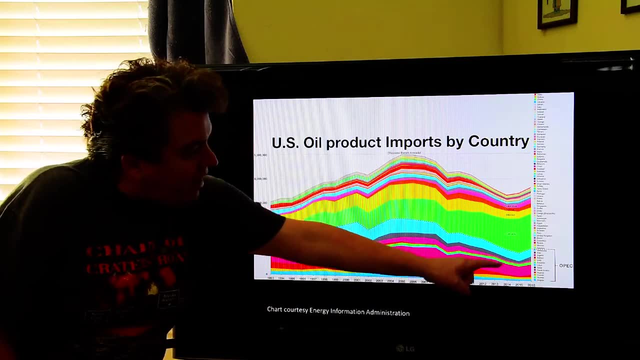 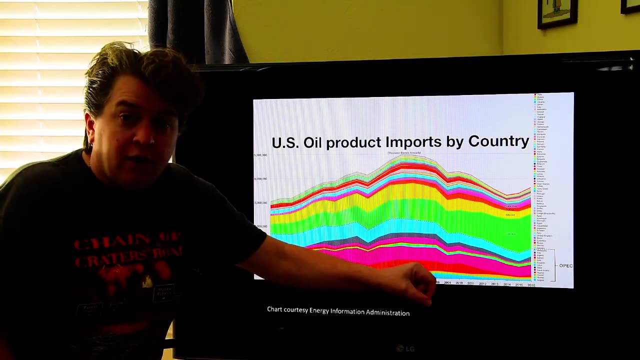 dashed line, that's the imports that come from OPEC, And then, above it, are all the other countries And of the other countries, actually of any country. the US gets most of its oil imports from Canada. Other countries that are major suppliers of oil do include Saudi Arabia and Mexico. 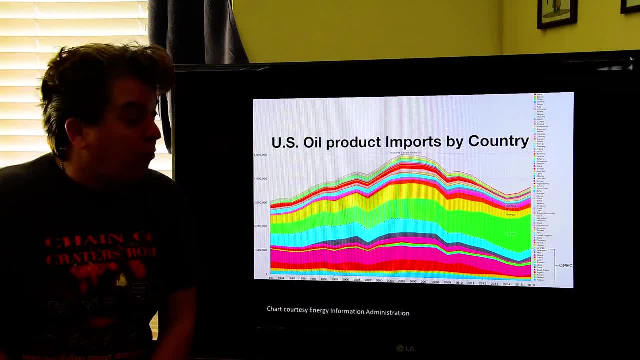 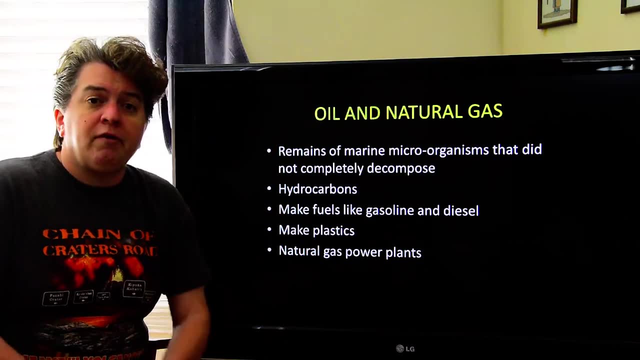 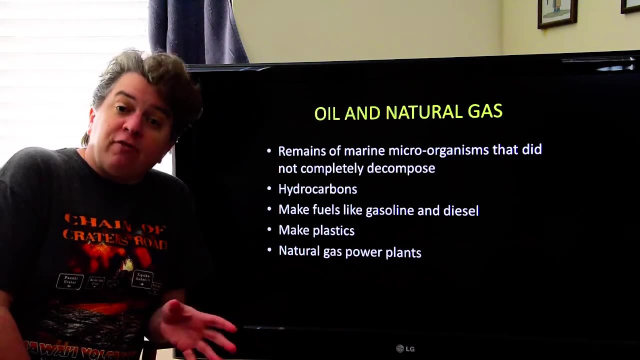 But anyway, Canada is the country we get most of our oil imports from. But let's take a look at how oil ends up forming and how we get all these different oil deposits around. Well, oil and natural gas are fossil fuels, So they're the remains of fossil fuels, And 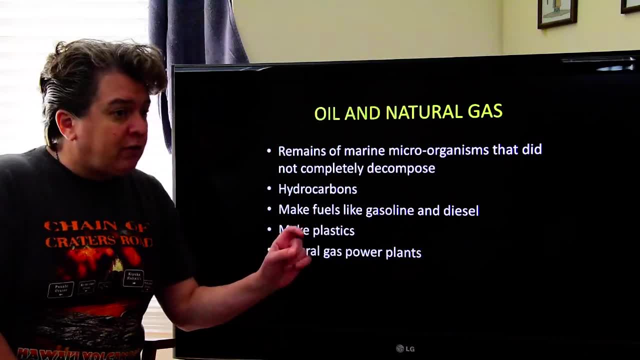 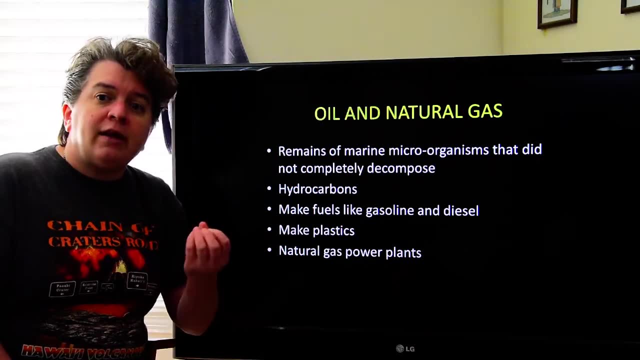 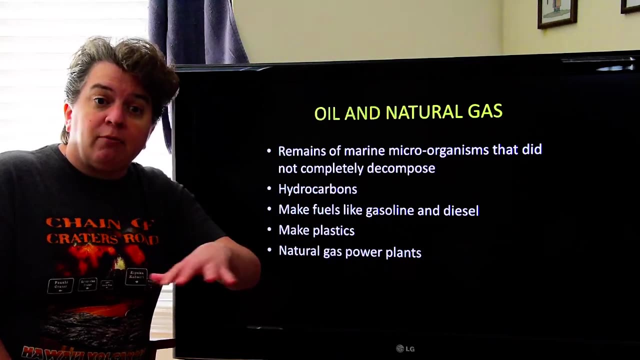 in the case of oil and natural gas, it's the remains of marine microorganisms, And these things did not totally decay after they died. So basically, we're talking about the plankton, all those little plants and animals that float around in the world's oceans. Eventually, 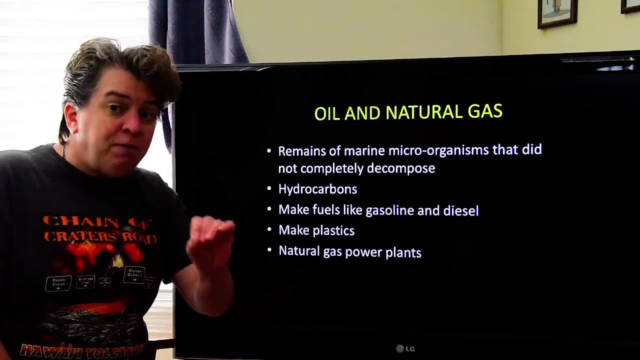 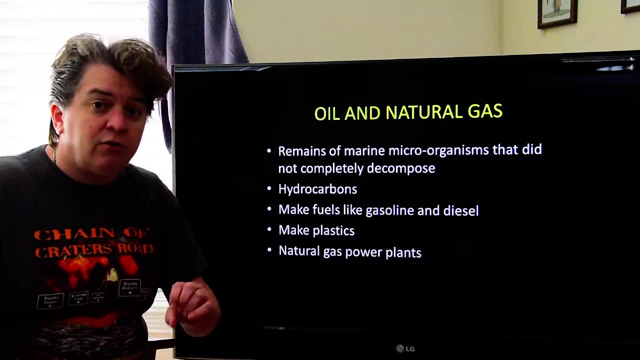 they die and they sink to the bottom of the sea And if the conditions are right down there, they won't completely die. They won't completely die. They won't completely die, They won't completely decompose And they could get turned into crude oil. Now that 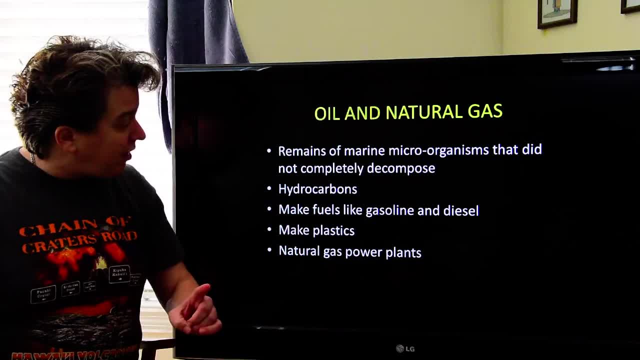 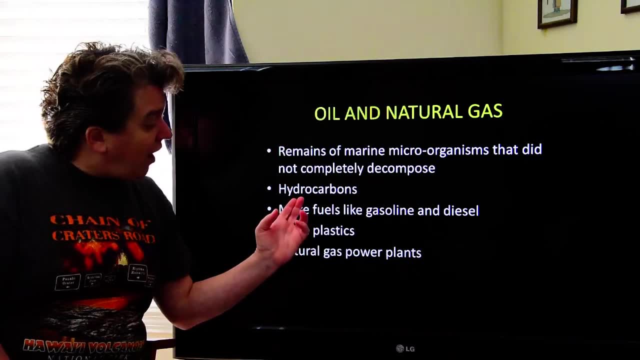 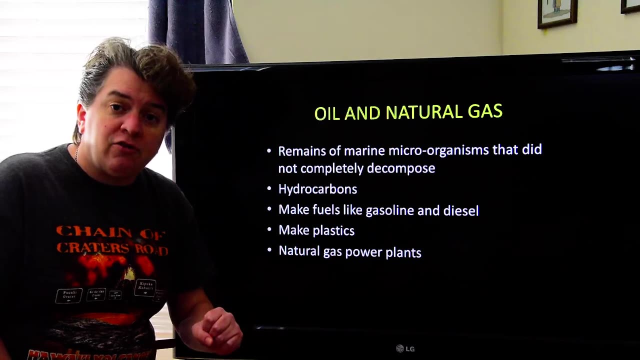 doesn't always happen. You need those perfect conditions for that to happen. Now again, these are going to get altered And they're going to turn into hydrocarbons. then Hydrocarbons are long chains of carbon atoms with hydrogens attached to them. It 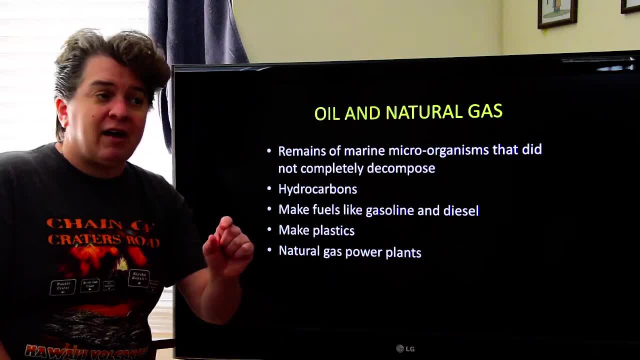 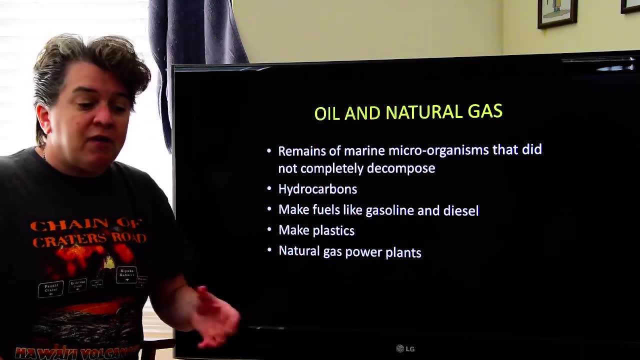 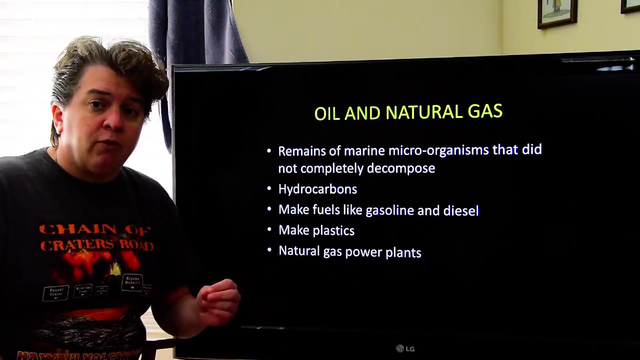 can be as small as one carbon with four hydrogens attached to it, Or it can be as long as hundreds of carbons long with hydrogens attached, But these are hydrocarbons that were created from those ancient marine microorganisms. Now what we do with crude oil is we can refine it and turn it into fuels like gasoline and 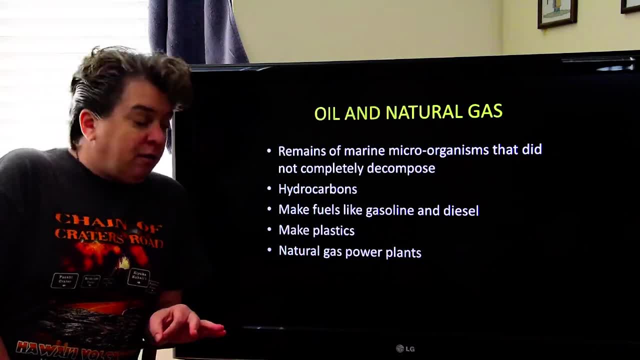 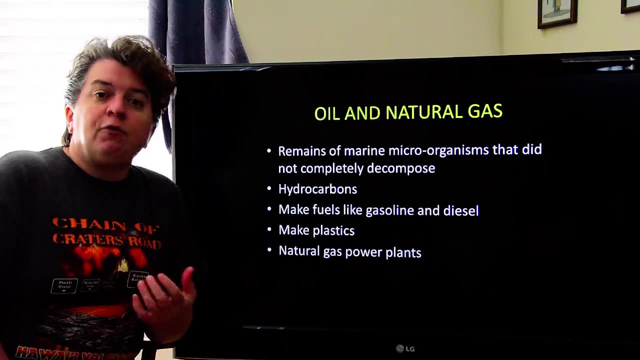 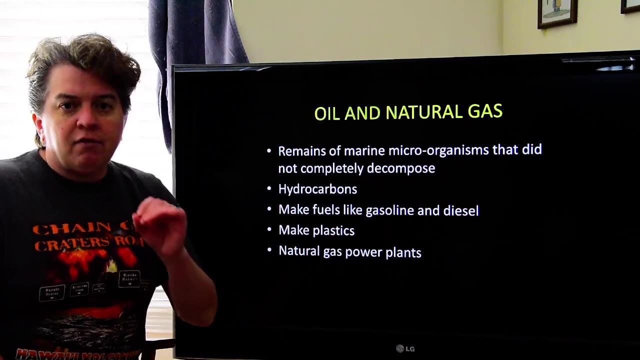 diesel, But it's used for many other things, including things like plastics. So if you had a plastic water bottle or if you wear glasses, you have plastic lenses in your glasses. Food is often packaged in plastics And this is why, when the price of oil goes up like 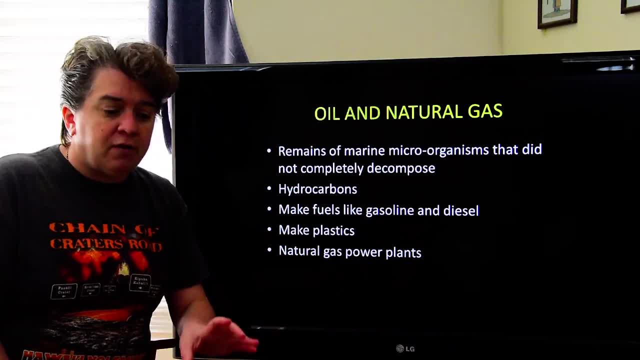 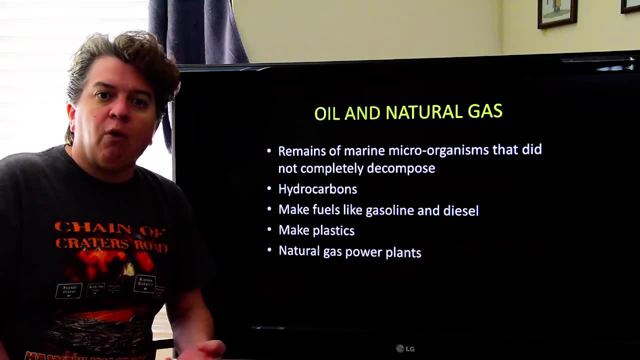 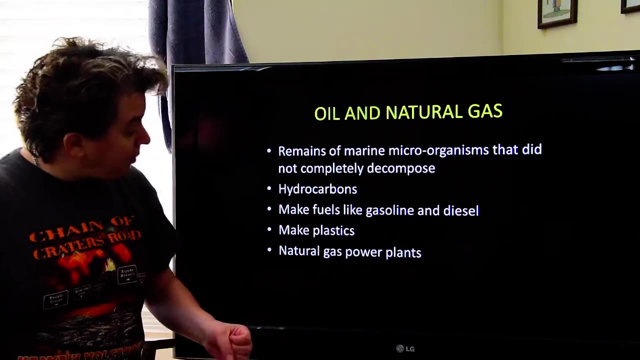 the price of almost everything goes up, because it's not just the cost of the fuels for transportation, It's also all these many things that are made from the oil, the hydrocarbons. that increases the price, including things like the packaging. Now, the other thing that we use this for are 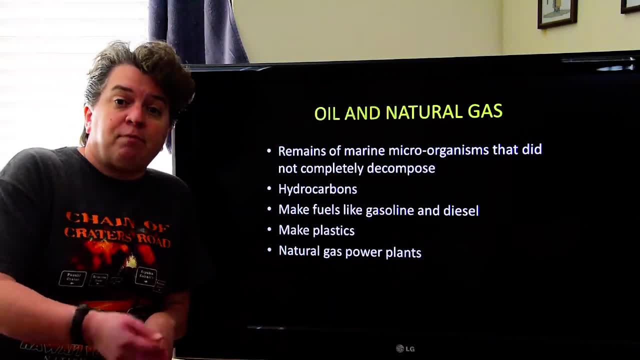 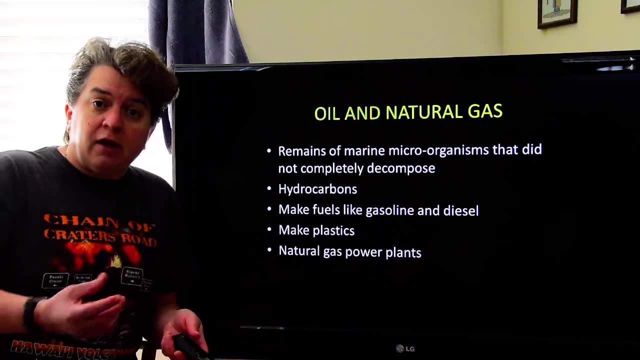 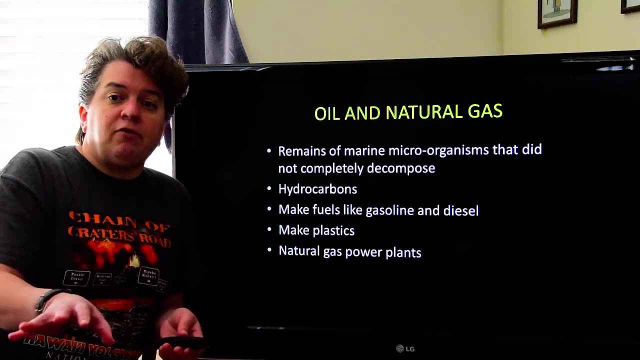 natural gas piles And in a natural gas power plant they burn natural gas. The natural gas heats water. The water turns to steam. The steam turns a turbine that turns a generator that creates electricity. And in this class, you just need to know, we need to spin a turbine to make. 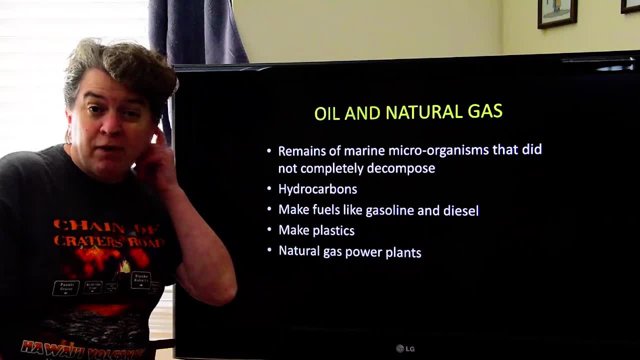 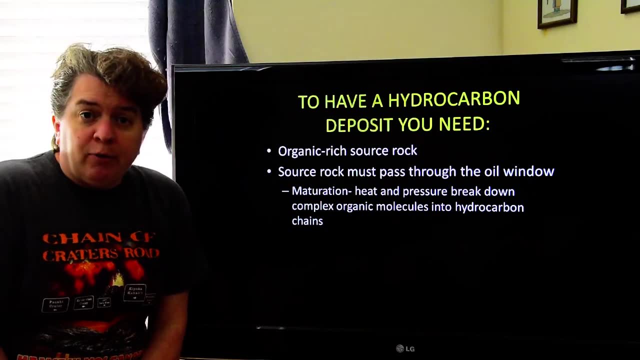 electricity. If you're interested in how and why that happens, take physics. All right, so let's look at what we need to have a hydrogel. Let's look at what we need to have a hydrocarbon deposit, because, I said, it doesn't always. 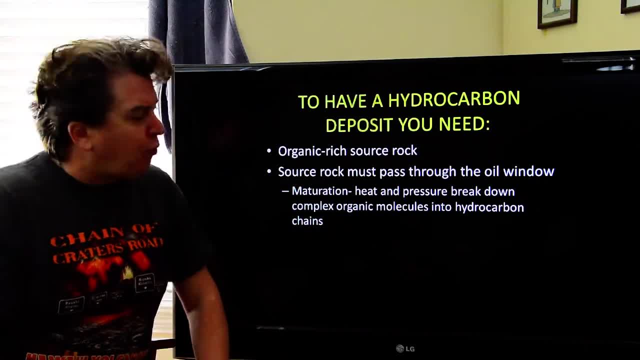 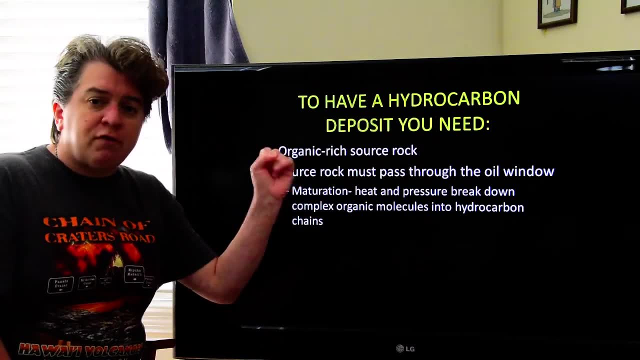 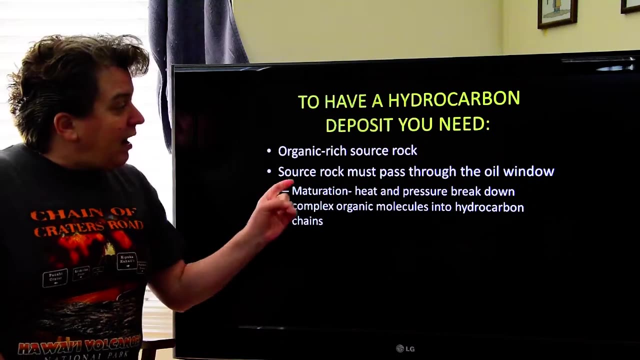 happen. You need these special conditions for it to happen, And you basically need kind of four things. First of all, you need an organic-rich source rock, right, You need that organic material to turn into your crude oil, And this organic-rich source rock must. 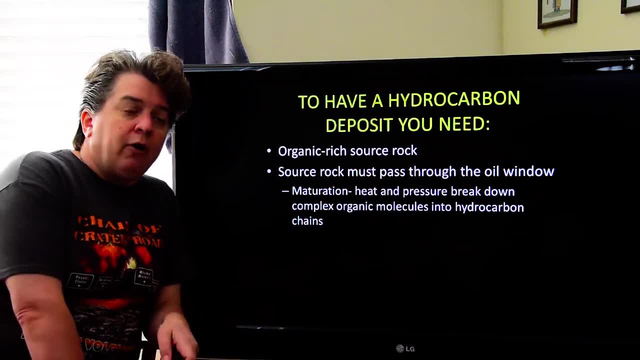 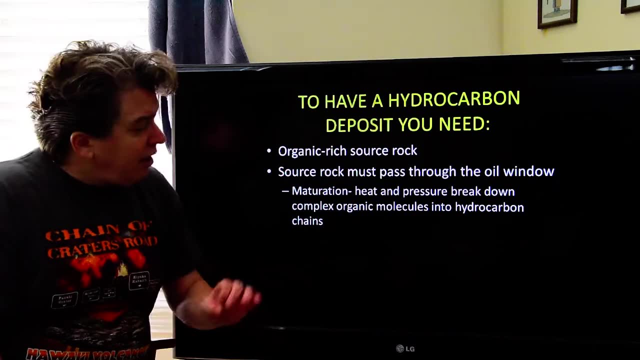 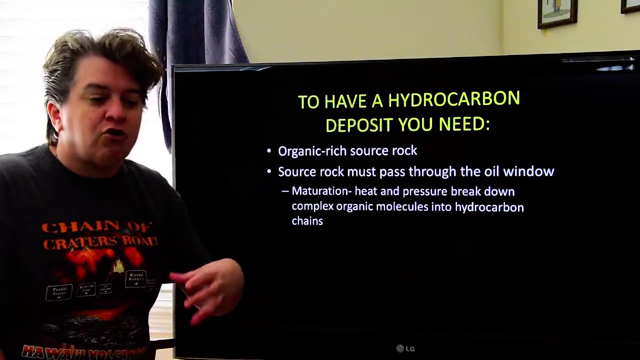 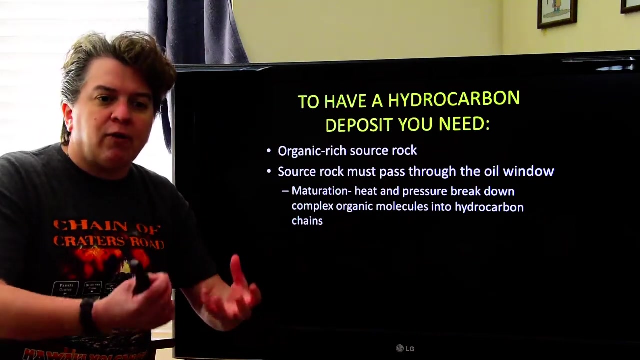 pass through something we call the oil window. The oil window is the temperature and pressure conditions needed to break down those complex organic molecules in the organic source rock and turn them into these hydrocarbon chains. And this process of having the right temperature and having the right pressure to do that is called 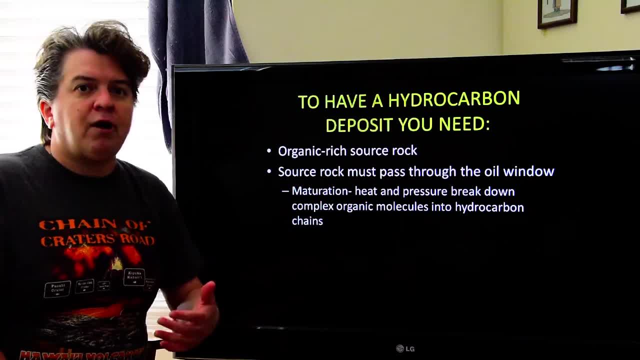 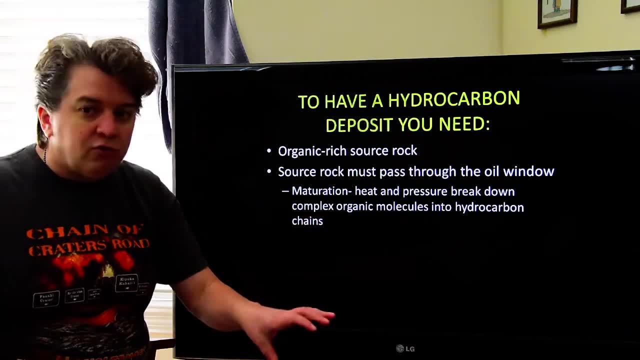 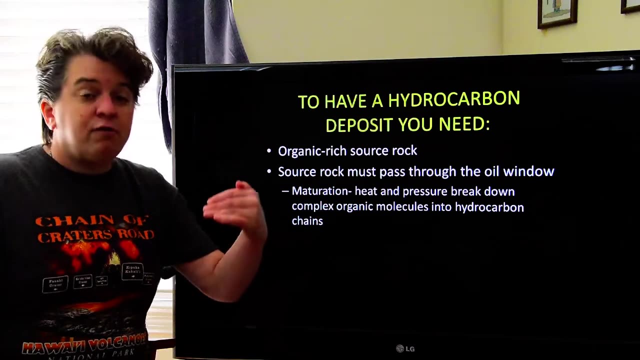 maturation. So if you ever hear someone talking about the maturation of the oil- or they're talking about it being turned from the complex organics into the crude oil And the perfect conditions we call the oil window, If it gets too hot it's going to burn away the hydrocarbons. If it doesn't, 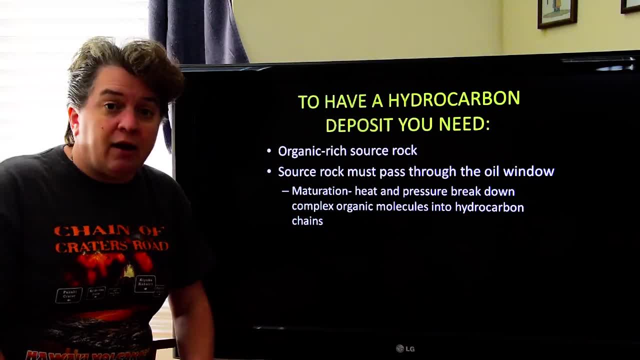 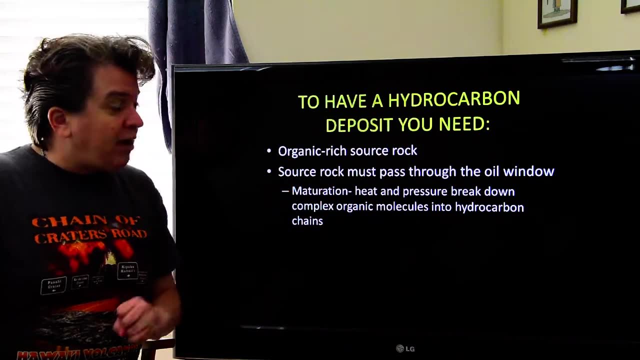 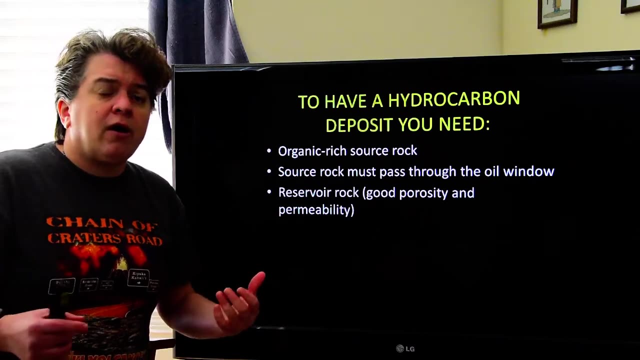 get hot enough, it's just going to stay as complex organic molecules and never get turned into oil. So we need an organic-rich source rock. We need it to pass through the oil window. We also need a reservoir rock, And this reservoir rock is a place where the oil is going to sit and it's going to 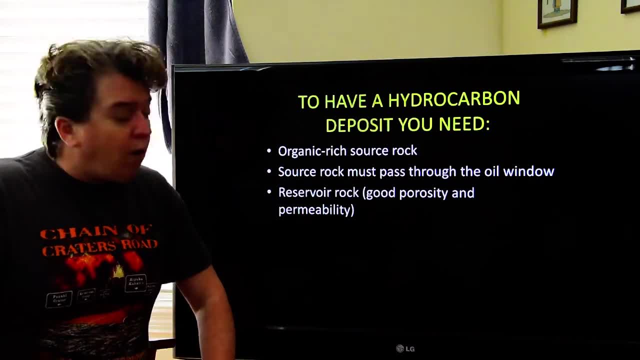 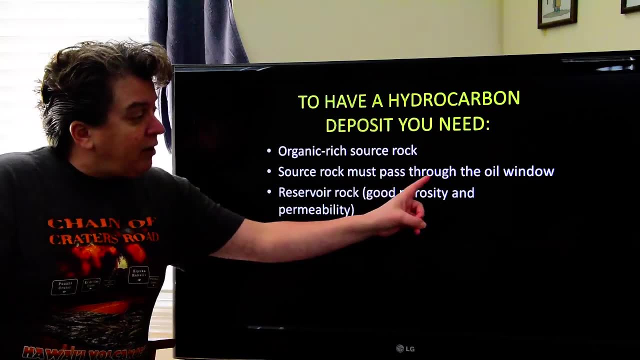 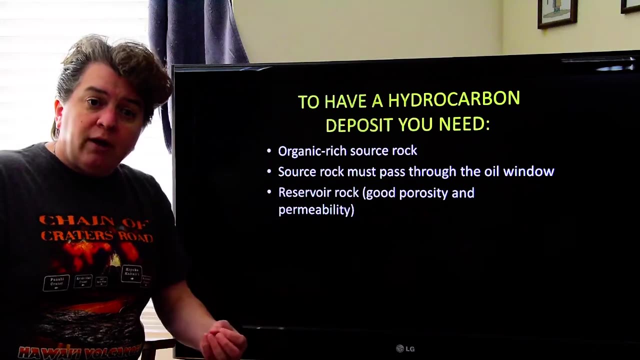 accumulate and get stored until we want it, And so your reservoir rock should have good porosity and good permeability, Because we want it to hold a lot of oil right. That's the porosity: lots of open space, And we want to be able to drill into that rock and have 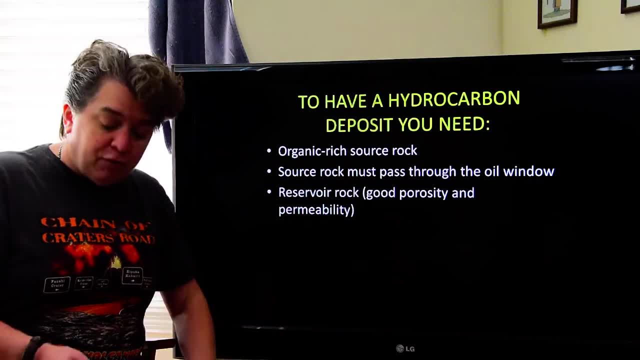 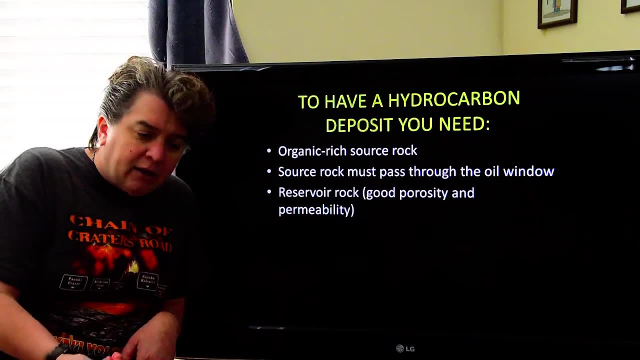 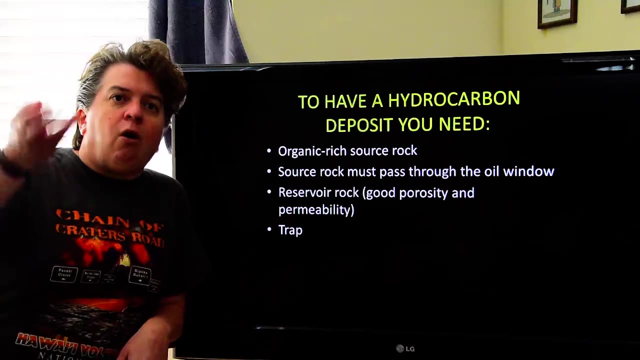 the oil flow from the rock into our well. That's the permeability. But we need one more thing, And this is because oil is low density and it likes to rise upwards as far as it can go- And if it could it would rise all the way to Earth's surface. But we don't want it to. 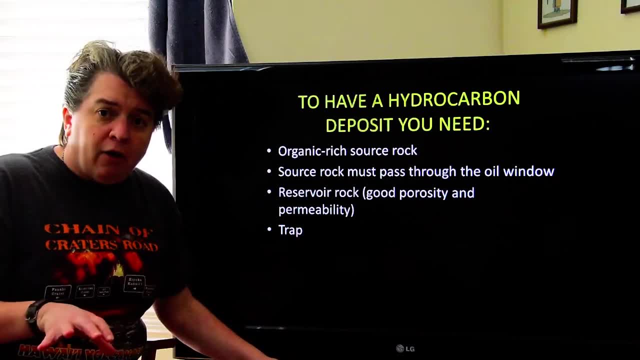 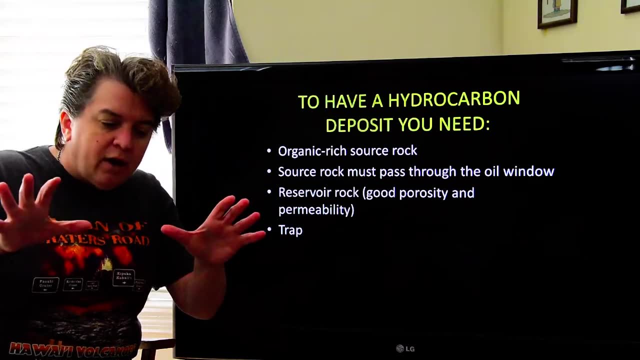 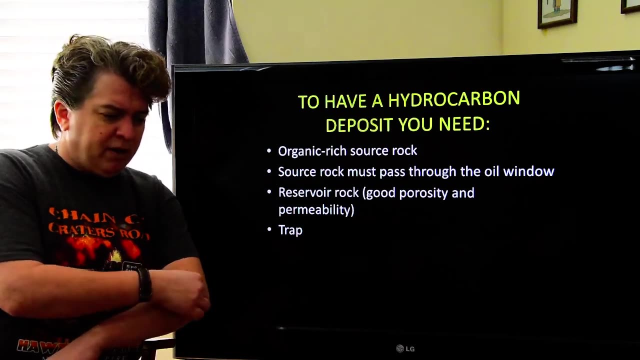 do that. We want to keep it underground, So we need a trap, We need something impermeable to hold that oil underground. You might be asking: well, why do we want it to stay underground? Wouldn't it be a lot more convenient if it? 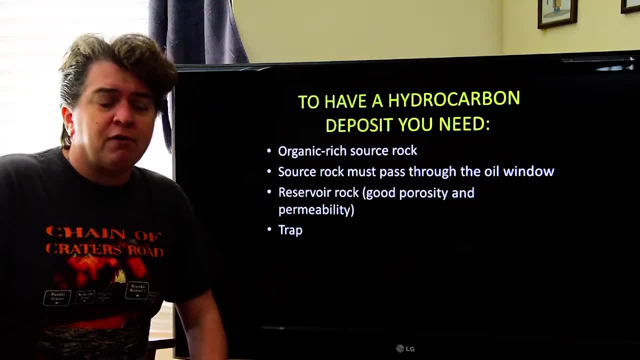 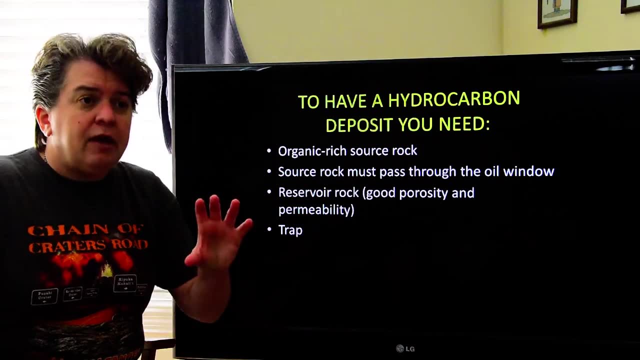 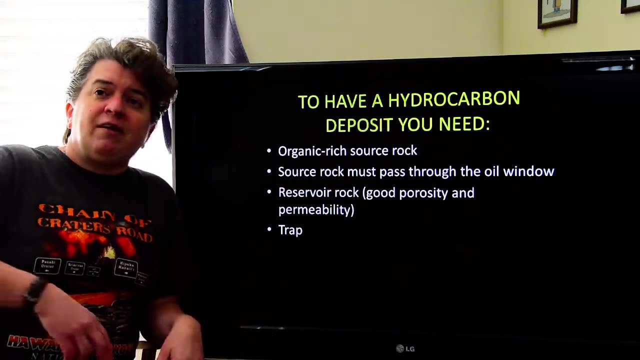 just flowed to the surface and we could like catch it in buckets or something. Well, the problem is that when oil gets to Earth's surface, the smaller, shorter hydrocarbon chains tend to volatilize, which means they basically disappear off into the atmosphere. 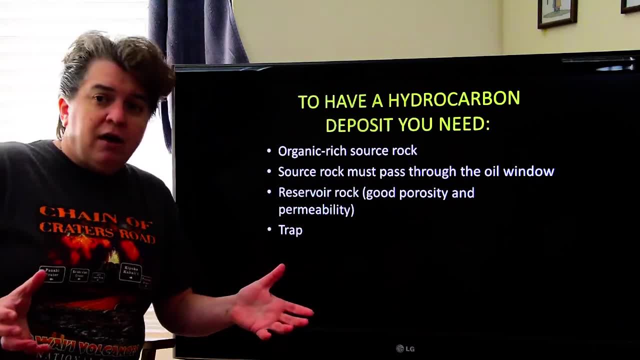 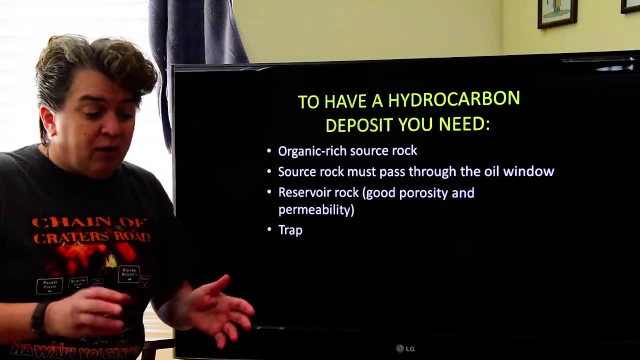 And all we're left with are longer hydrocarbon chains. So if it makes it to Earth's surface, we actually are losing some of the hydrocarbons And we're in fact losing some of the really good part of the hydrocarbons. So we want 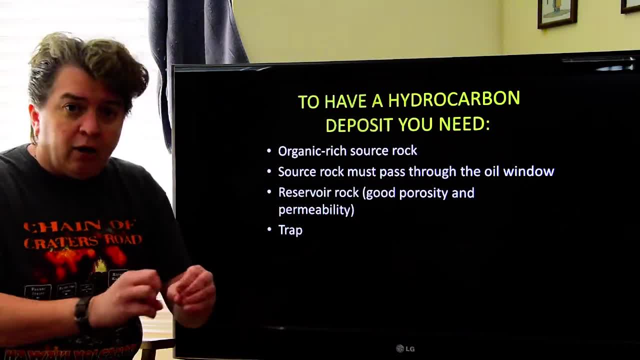 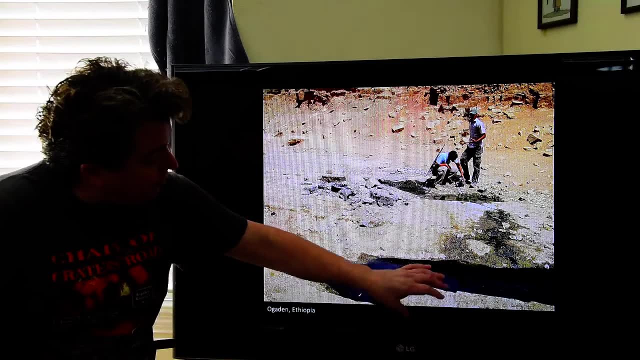 it to stay underground until we are ready to use it. So if you do not have a trap, it'll come to the surface, it'll flow like this on the surface and you're going to start losing some of those hydrocarbons to the atmosphere. So let's look. 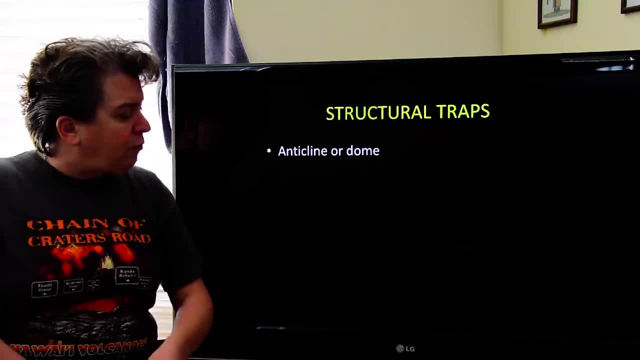 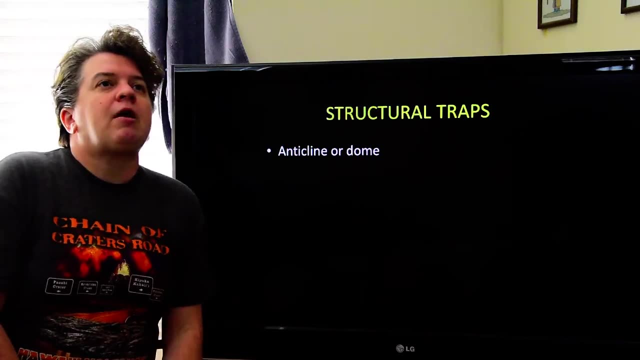 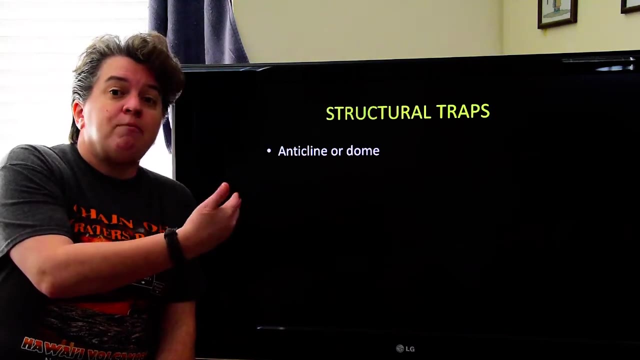 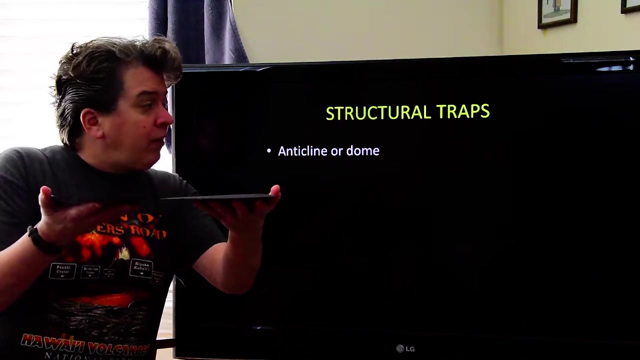 at a couple of traps or a few different types of traps. We're going to start with ones that are called structural traps. Now, structural traps are created by your rocks are originally horizontal because your oil deposits are found in sedimentary rocks, and sedimentary rocks originally form in the horizontal state. Well, the thing is you. 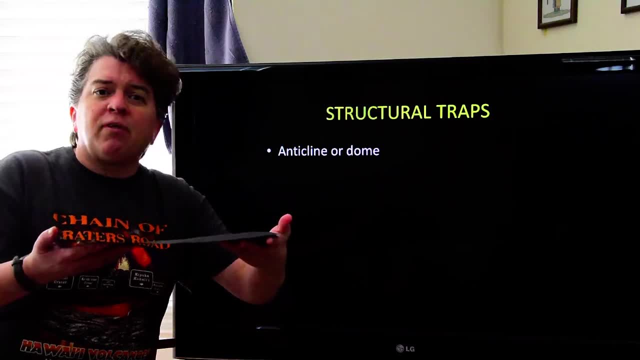 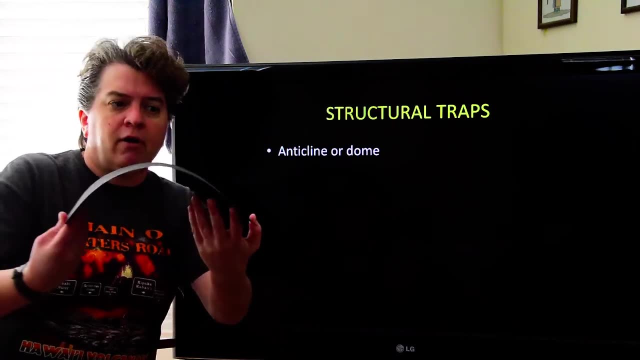 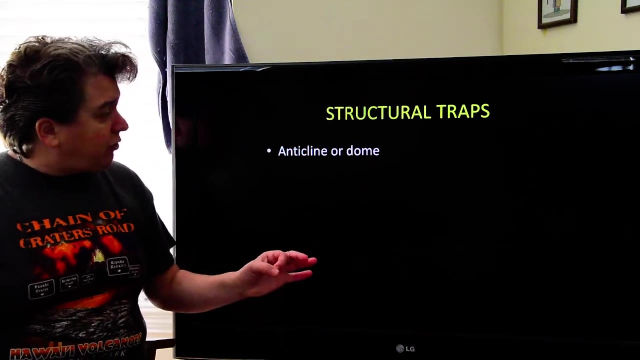 can get geologic structures forming because of you know, the plates moving around and stuff like that, and when that happens, the rocks can get bent upwards or downwards or they can get tilted in different ways, and that's a geologic structure and a classic structural trap is an anticline or a. 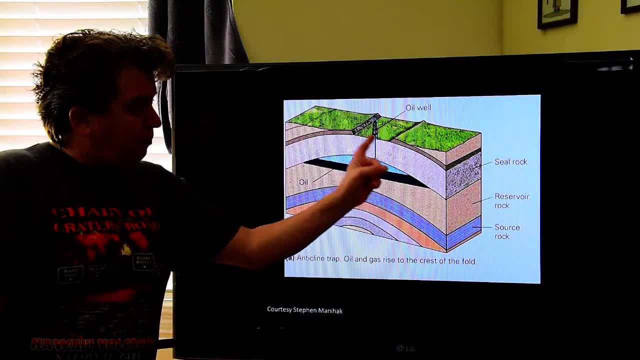 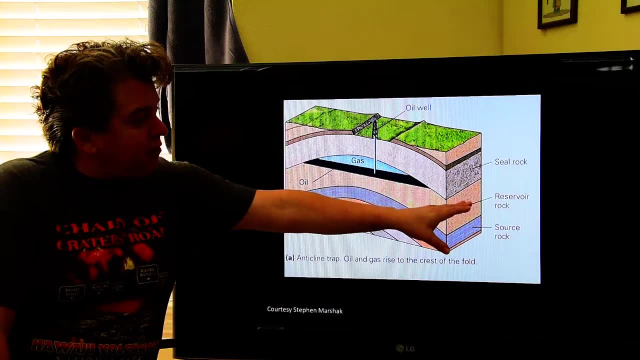 dome and it is arched upwards like this, and so what we're seeing in here? we have some organic, rich source rock. down here there's our reservoir rock. you can see it on the right and I'll zoom in a little bit and I'll show you. 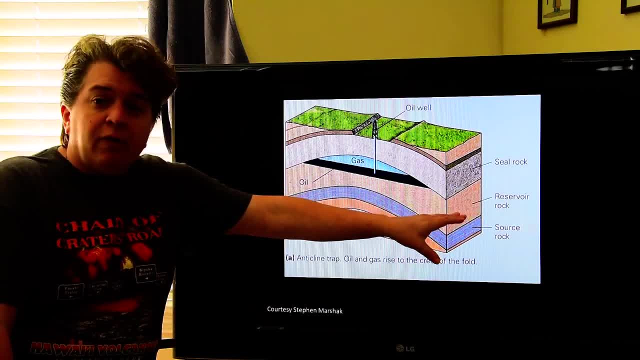 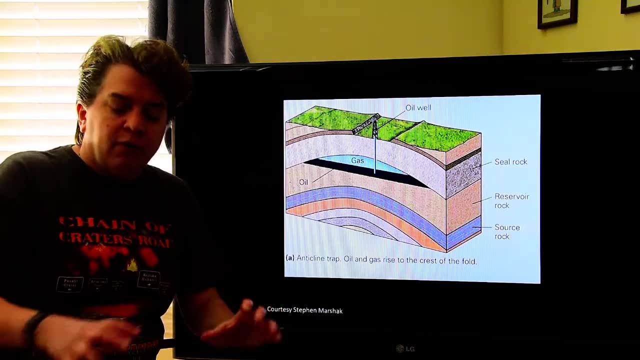 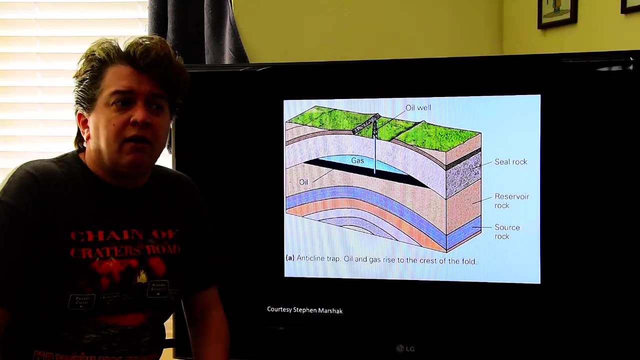 with good porosity and permeability. A classic reservoir rock is a nice sandstone with lots of open space in it. And then we have this thing that's called the seal rock. Well, that seals the oil underground, So that's an impermeable rock And oftentimes that's something like shale. 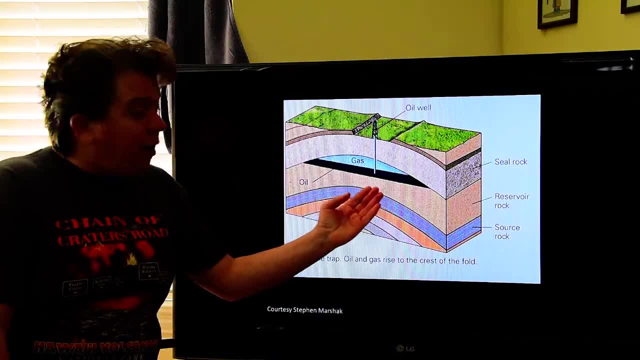 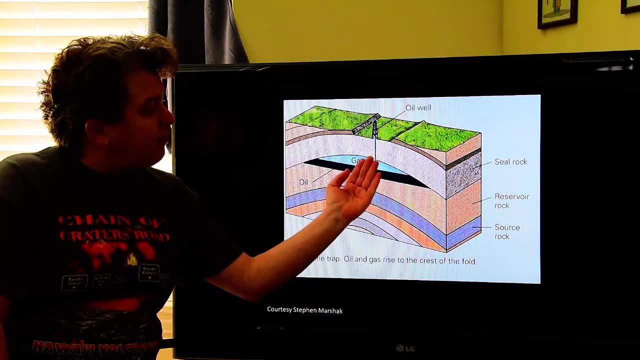 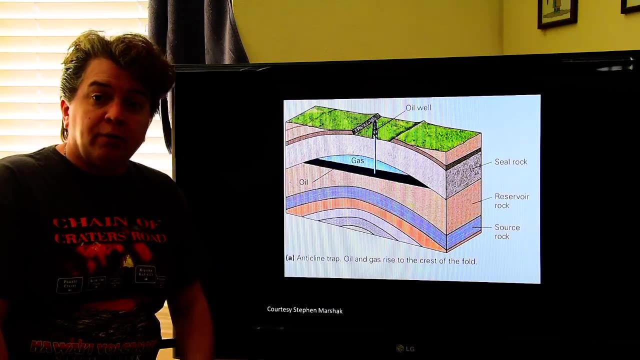 Shale is frequently impermeable. So this oil then that's created. as the source rock passes through the oil window, it's going to rise upwards as far as it can go And it gets stuck underneath that impermeable rock And there's our oil deposit And what you will usually see in these, you'll see. 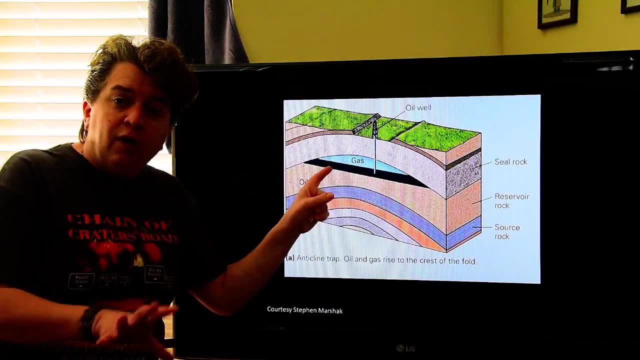 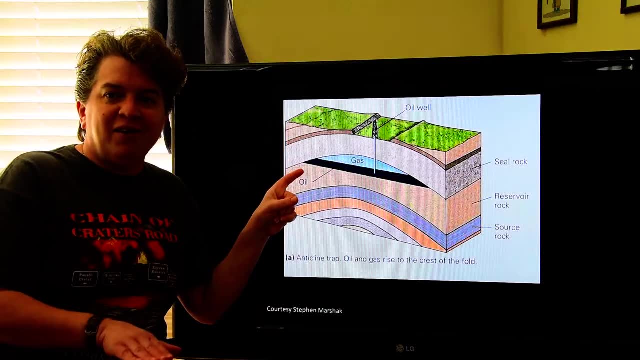 natural gas at the top, because that's the lowest density. Then under that you'll have your oil trapped in the rock And then underneath that you'll often- it's not shown on here, but you'll often have water, And it's usually. 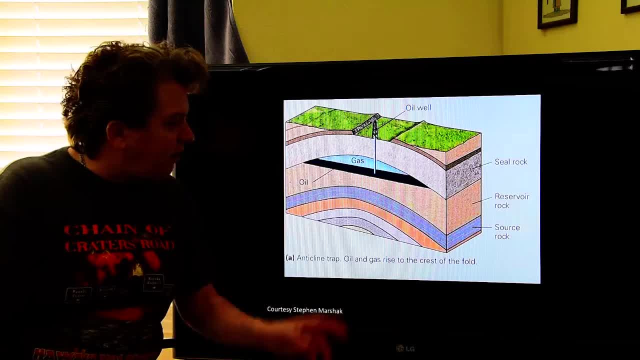 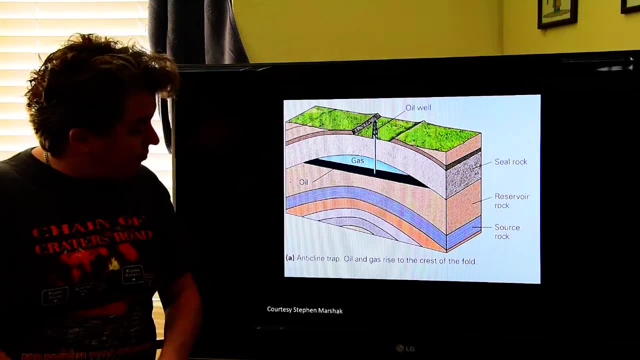 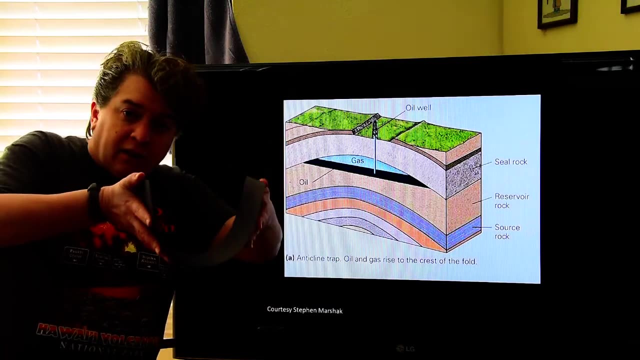 kind of really nasty, salty, sulfurous water, not really nice, but that's usually underneath the hydrocarbons And that's because it is denser than those hydrocarbons, And so that's our anticline. Now the reason: an anticline is a good trap, but a syncline is not. So if we bend the rocks like 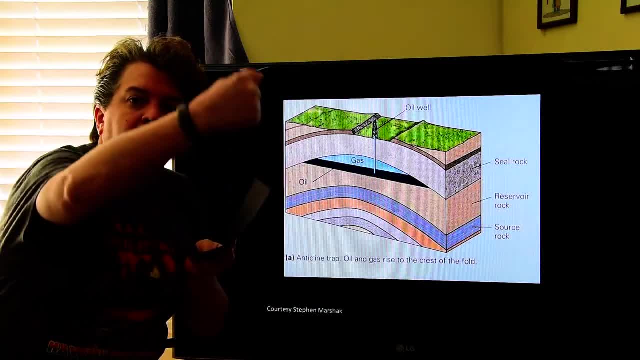 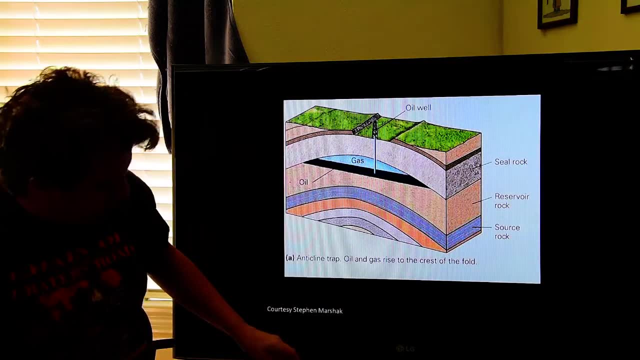 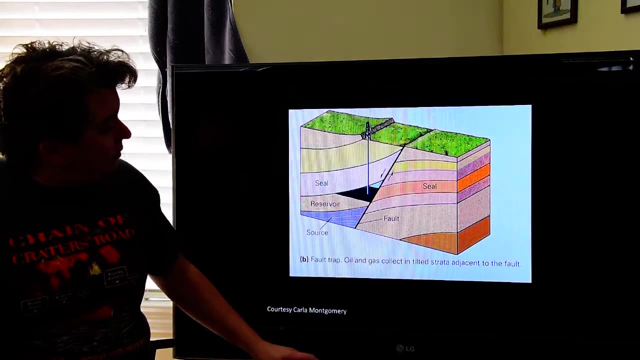 this. the problem is they'll just flow up and not get trapped. So we want this shape where the rocks or where the oil can get trapped In those rocks. Now another structural trap is a fault. So what we see in this fault, we've had movement right. 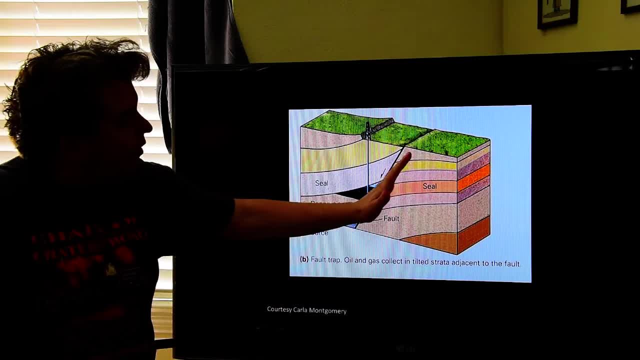 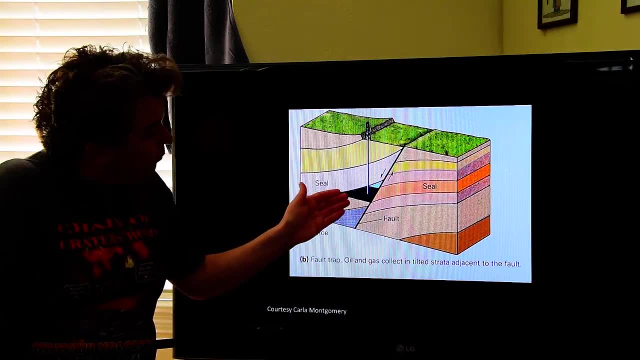 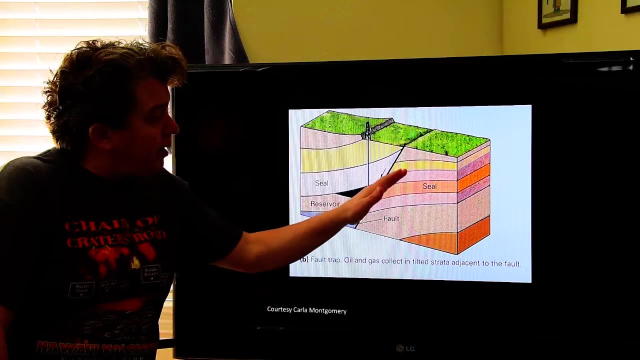 Right, there is the fault. Here's our reservoir rock, And then on the other side of the fault we have impermeable rocks. So again, the oil can rise up as high as it can go And it will get trapped underneath and next to the rock And that's why it's called an anticline And that's 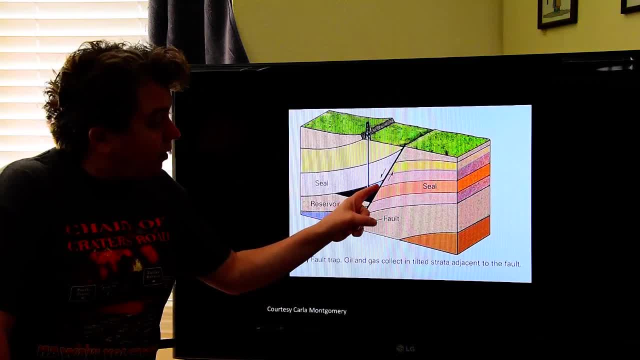 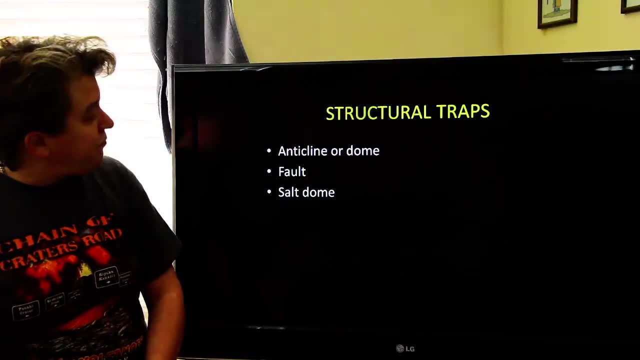 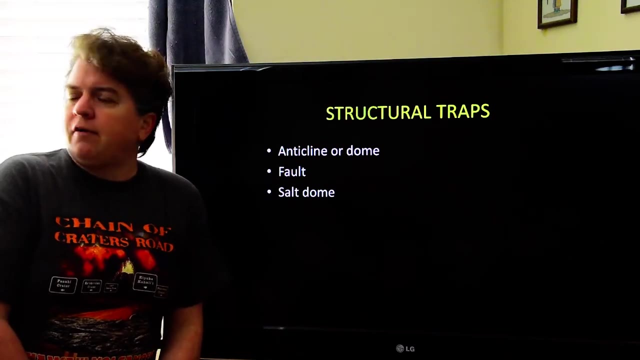 because of these impermeable rocks, And so we're going to see our natural gas at the top, our oil and then kind of that nasty water underneath that. Now, the last of the structural traps I would like to go over is a salt dome, And I want to go over 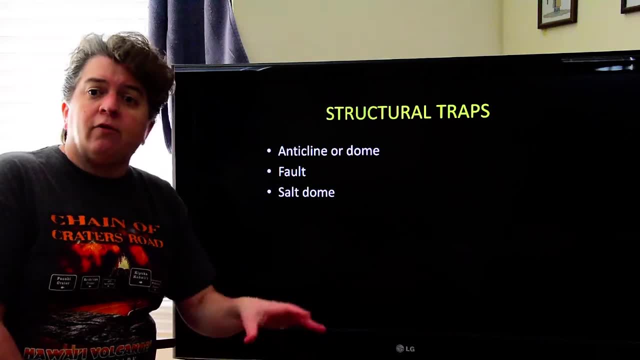 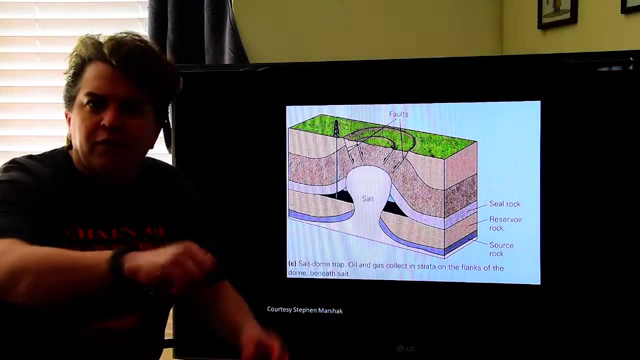 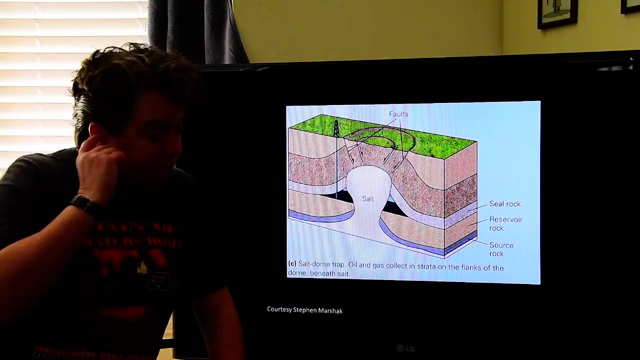 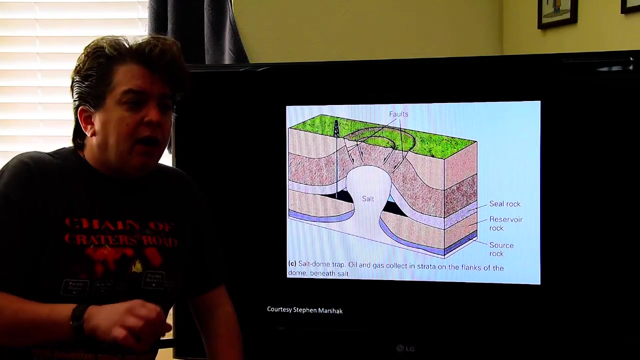 these because a lot of the oil that's found in this part of the world, around Houston, is actually found on salt domes- Salt, basically, rock salt. the stuff that you put on your dinner is a really unique rock type. First of all, it is very low density compared to other rocks. Secondly, when it is under pressure, it becomes 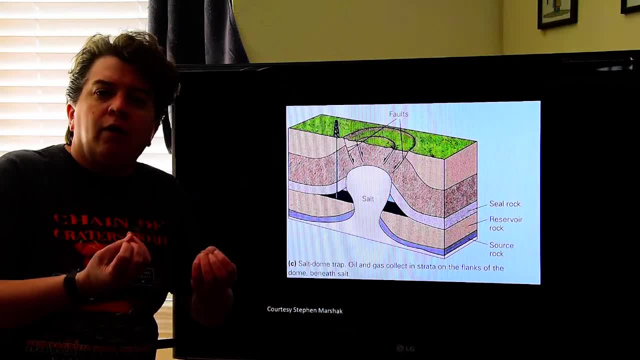 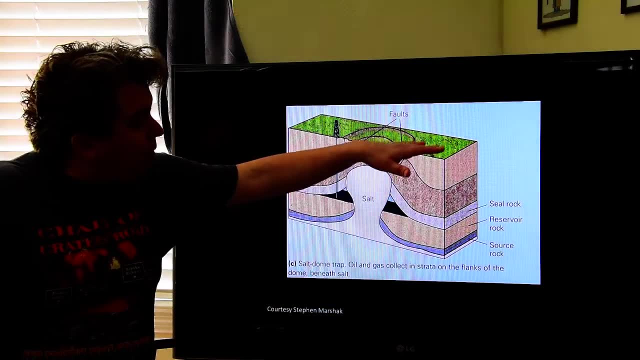 ductile, That means it can flow, And so what happens when we have a layer of salt buried under a whole bunch of rock? we're going to have a lot of salt, And that's because we're going to have a lot of rock. 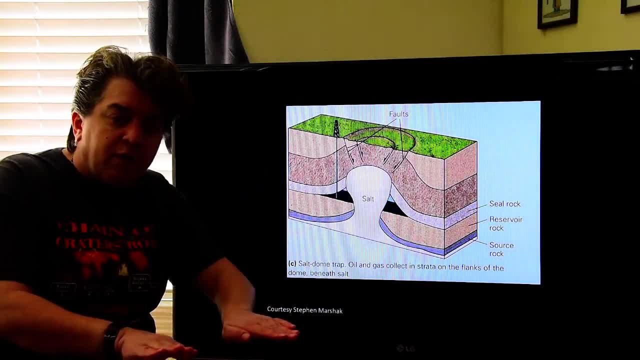 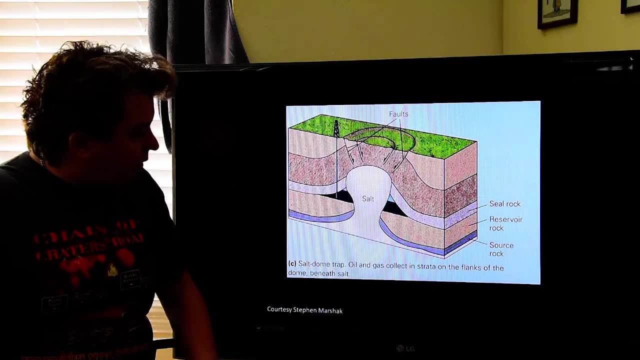 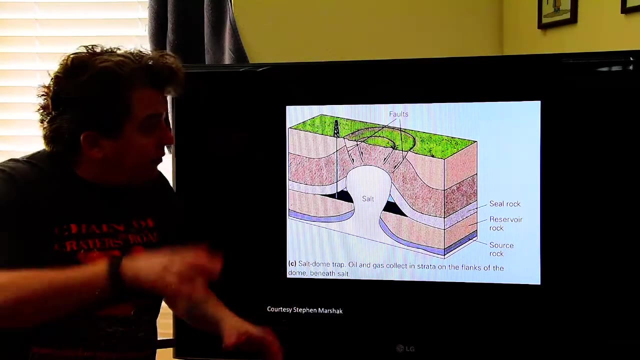 buried under a whole bunch of other rocks. Those rocks are pushing down on the salt and the salt starts flowing And because it's low density, it's going to start flowing upwards And this creates a salt dome, because it's going to start pushing the rocks above it kind of upwards, And salt also is going to be. 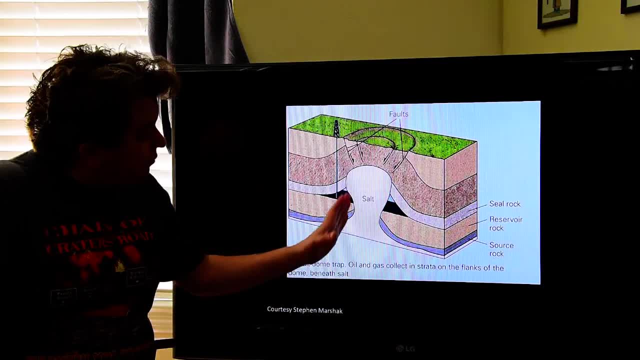 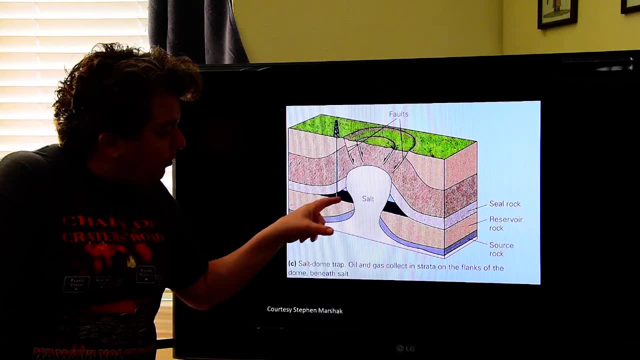 impermeable. So again, as the salt deforms and bends these rocks around it, as it's rocked, it's going to start rising. Well, we can have one of these nice, permeable and porous reservoir rocks And up against it. 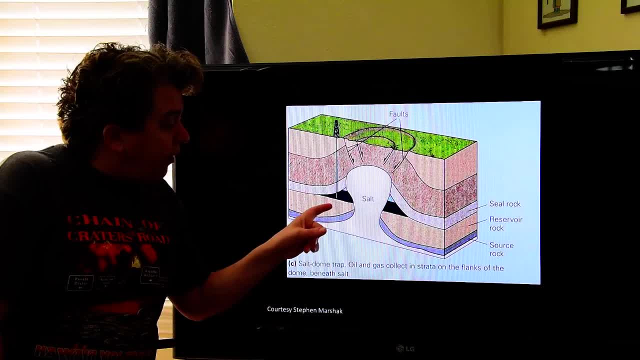 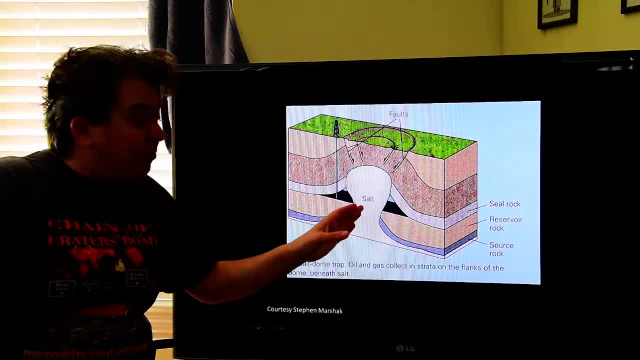 we're going to trap our natural gas and our oil And, yeah, we can still have some of that water down there Because, remember, I said it's really, really salty, So it's not going to be dissolving any of that salt, And so 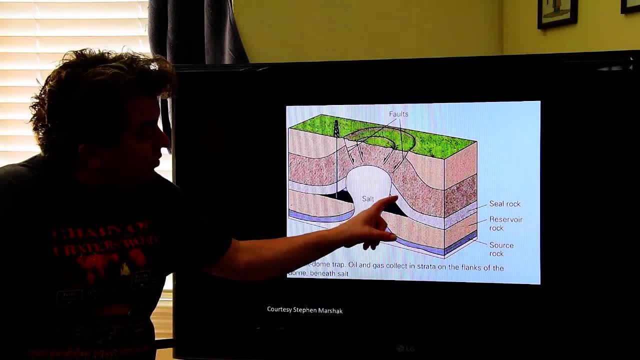 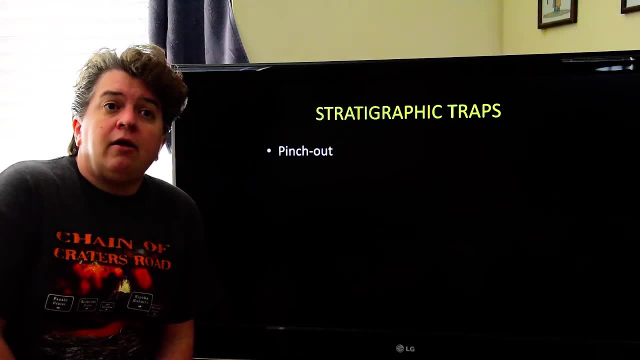 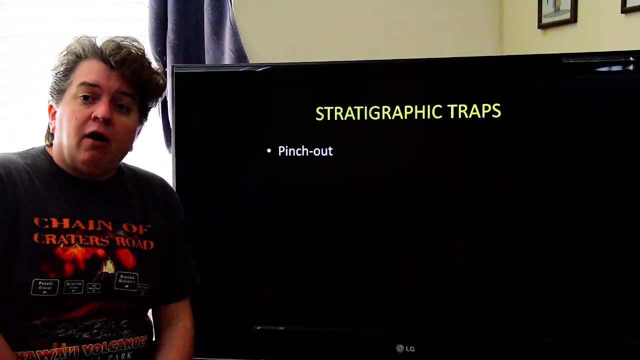 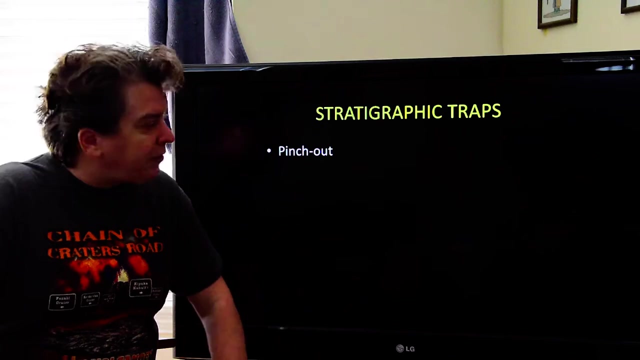 we're going to have these hydrocarbons trapped next to that salt dome And, like I said, that's found in many places in this area where they extract oil. Now there is another type of main group of traps for oil, And this is called stratigraphic traps. When we refer to this, 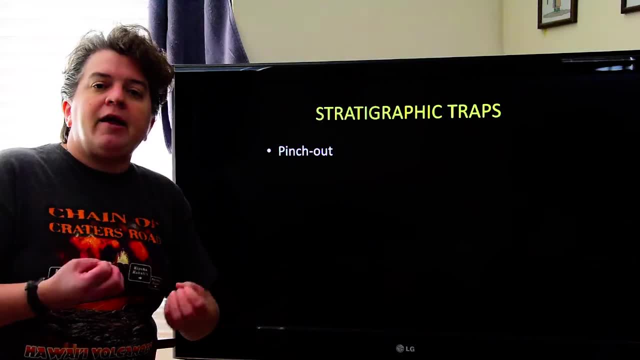 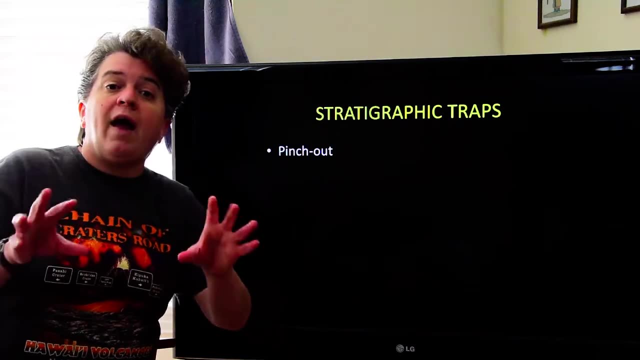 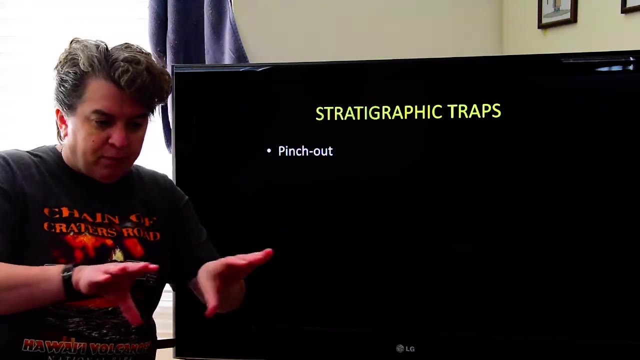 term stratigraphic, that means layers of rock. So there's simply some kind of characteristic in the layers of rock that was created When they were formed. that traps oil And that's what makes it different from structural right, A structural trap. the rocks were formed and then something happened to them afterwards, Like they got. 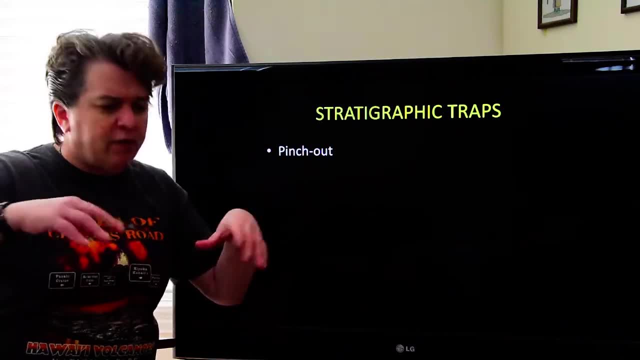 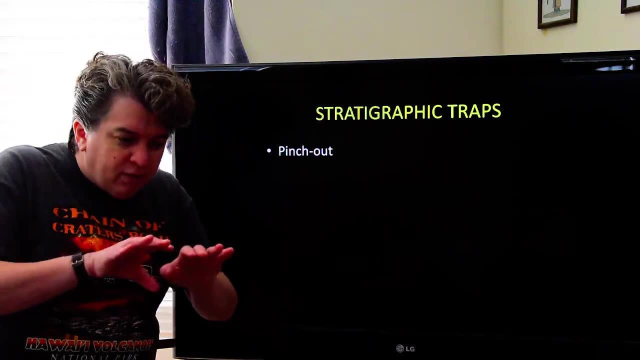 bent on that anticline, or they got broken on the fault or they got bent by the salt moving around after they formed And the stratigraphic traps. there's some characteristic about them when they formed that allows them to capture and trap oil. 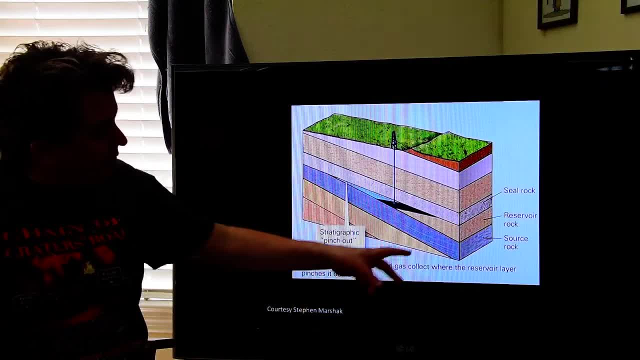 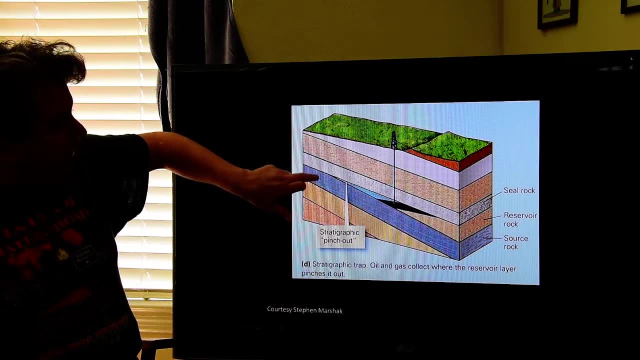 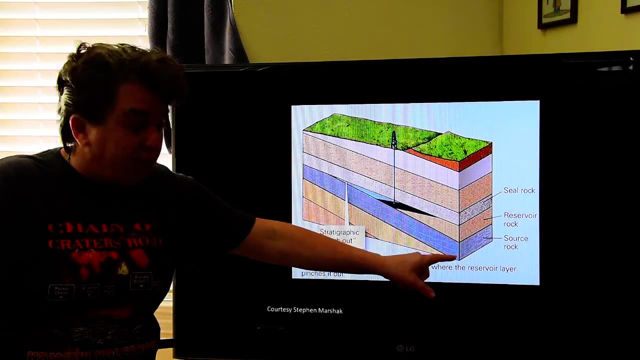 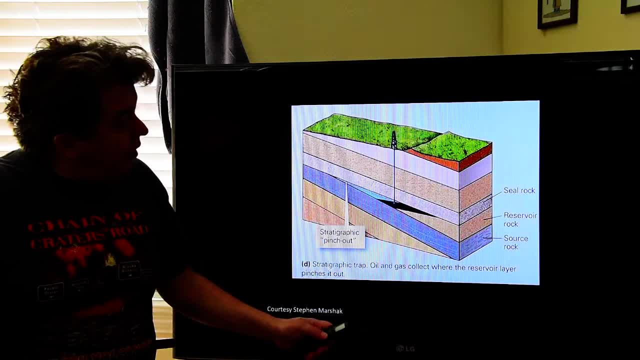 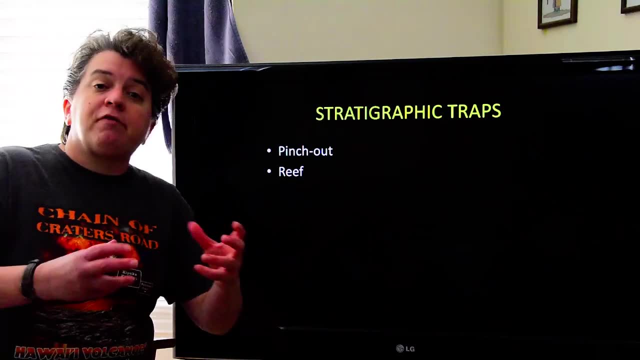 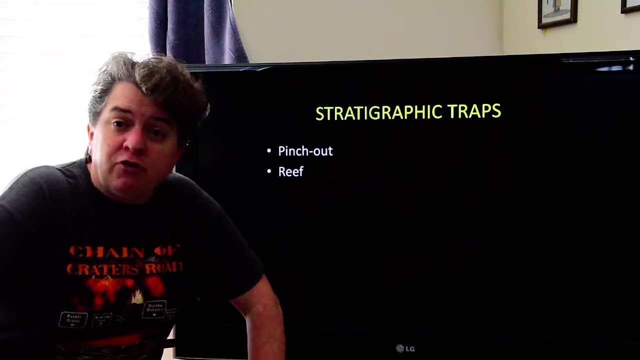 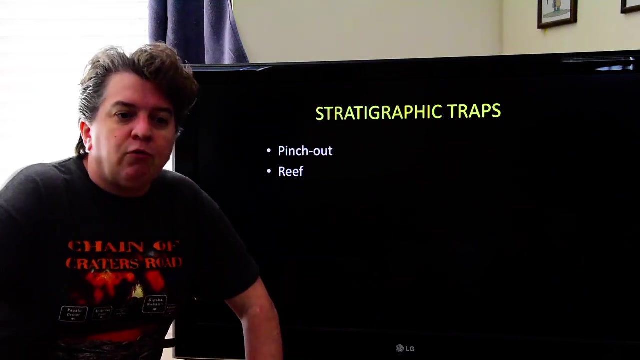 and then it's going to get stuck there. Another type of stratigraphic trap is a reef: Reefs- these growths of organisms in warm shallow seas have occurred throughout much of geologic history, or at least I should say throughout the past, like 550 million years of geologic history. And reefs, when these organisms are growing. there's a lot of open space in them. right, There's going to be a lot of porosity. Well, the reefs can eventually get buried under younger rocks, and those younger rocks might be impermeable, So you might end up with a reef trap. So originally we had this reef here growing. It got buried in these. 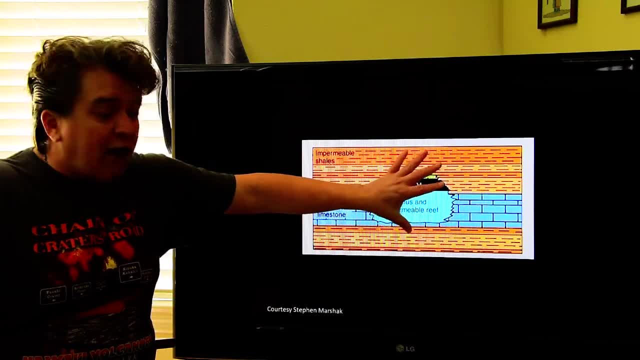 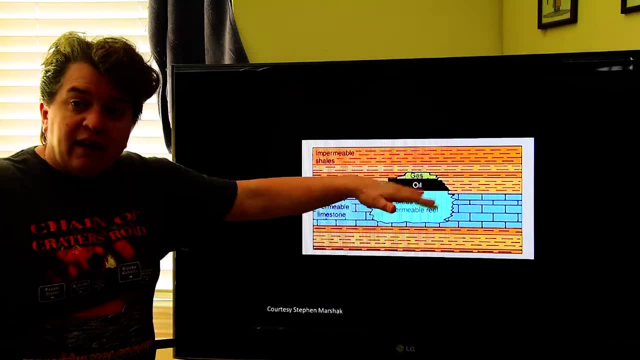 impermeable rocks which then can trap oil in there, And again you're going to have gas at the top, you're going to have oil under that and you'll usually have that kind of salty water underneath that. So those are some of the 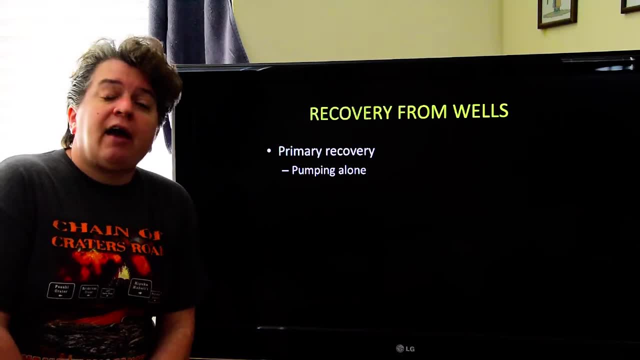 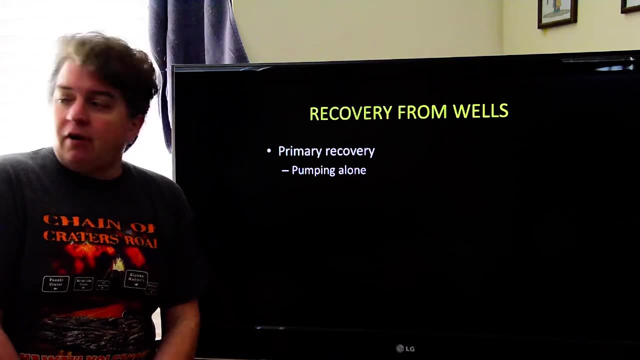 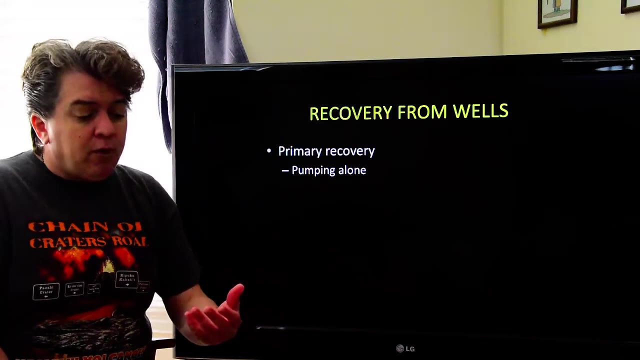 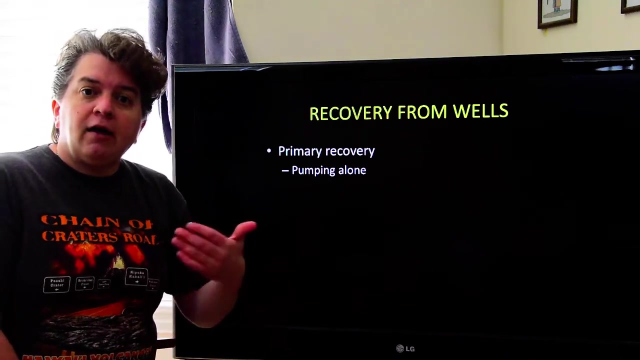 main kinds of traps That capture and hold oil for us to find Once we find oil, and there's a whole long way of all different kinds of techniques for searching oil and finding oil. but once we find a deposit of oil we have to get it out of the ground. How we do that is from a well 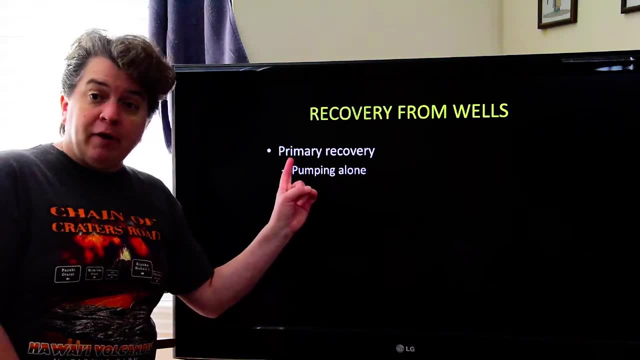 And the first thing you do- and that's what primary means right- The first thing you do is find oil in the open water过. Those are the types of traps that capture and hold oil for us to find And then, once we find oil- and there's a whole long way of all- 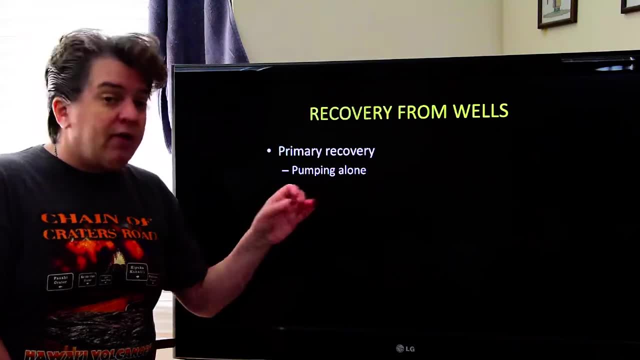 kinds of different techniques for searching for oil and finding it, but once we find a deposit of oil, we're going to have to get it. The first thing you do is simply going to drill a well and then pump the oil out, pumping alone. 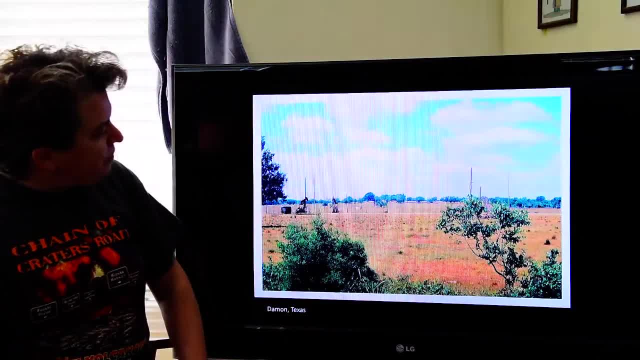 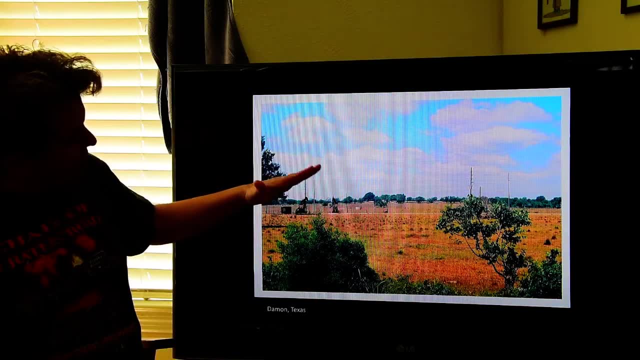 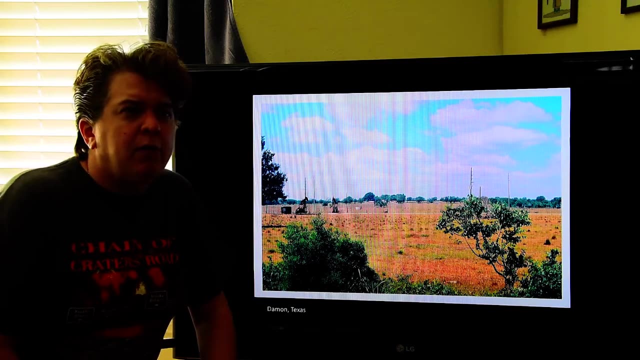 So that's primary recovery, the first technique used. And that's what these things are right, Those horsehead, these rocker pumps right there. every time it rocks upwards, it's pulling oil out of the ground. This is actually in Texas. This is the Damon Mound. 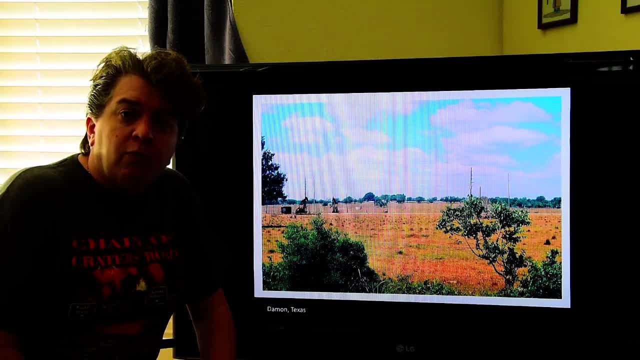 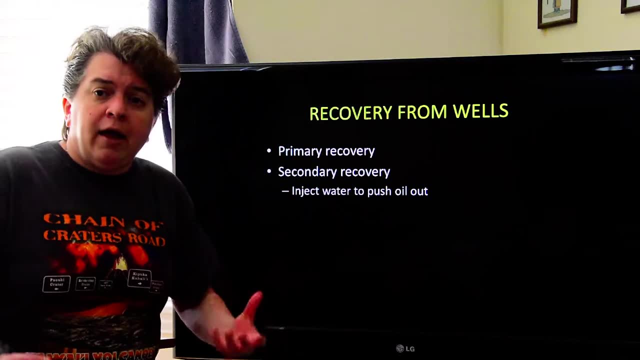 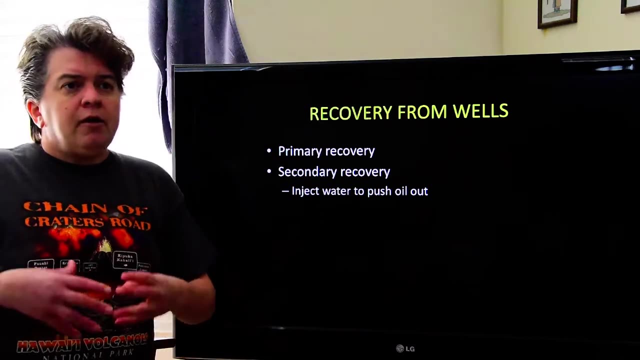 This is one of those salt domes where oil is extracted. Now, unfortunately, after a while, you can pump an oil reservoir and then it's not going to produce as much oil, And so you're going to need some help getting that oil out. 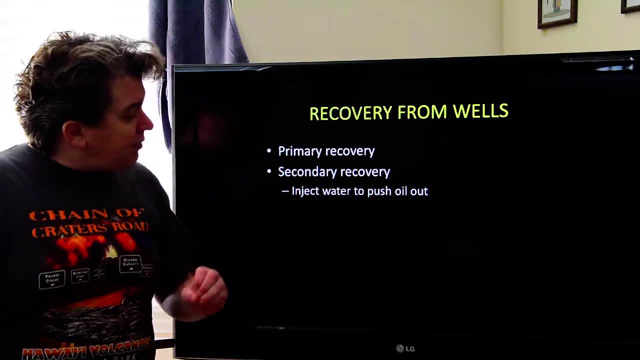 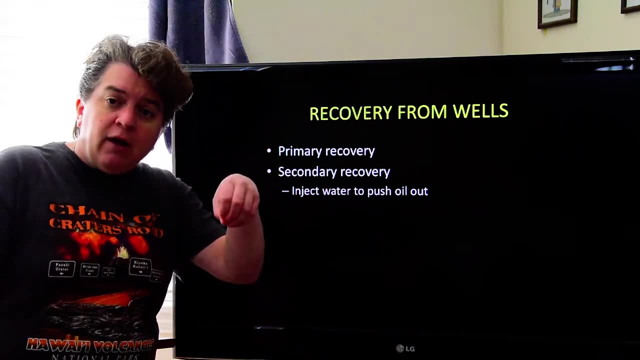 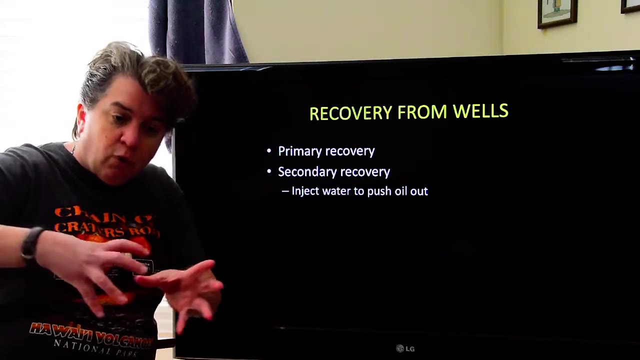 And this is where we come to secondary recovery. And secondary recovery is basically where we have one well where we're extracting the oil, but then nearby we have an injection well And what we do is inject water, push water into the oil reservoir. 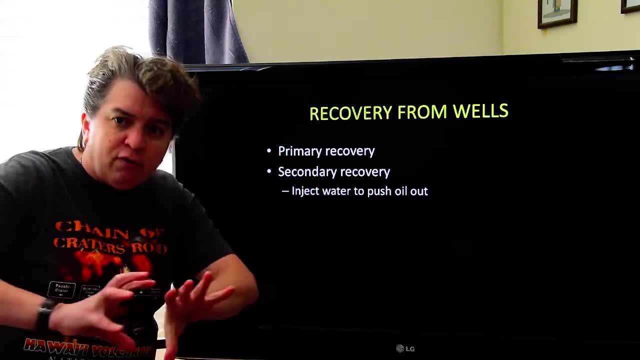 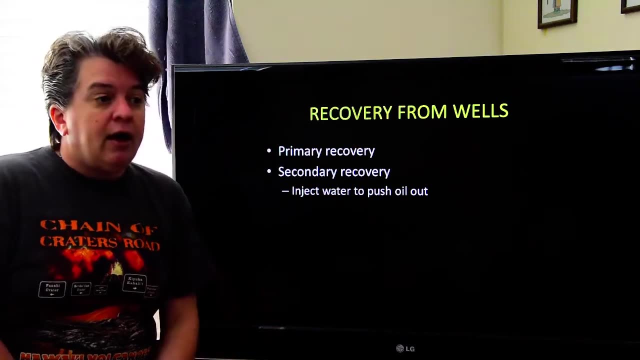 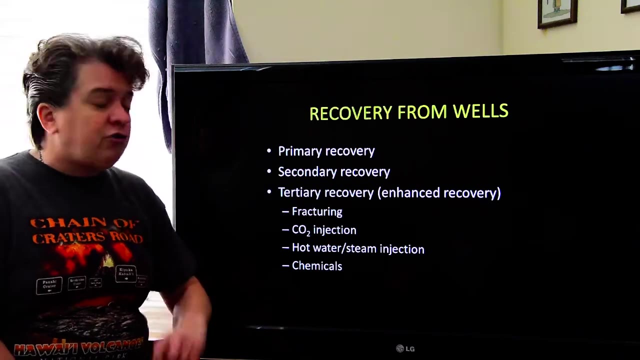 And as we push that water in, it basically flows through that rock and forces some more of the oil to leave the reservoir and get extracted. But eventually that sometimes doesn't work anymore, And so then we do tertiary recovery, or this is sometimes also called enhanced recovery. 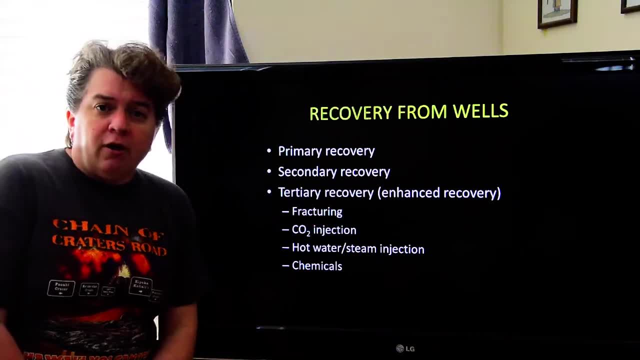 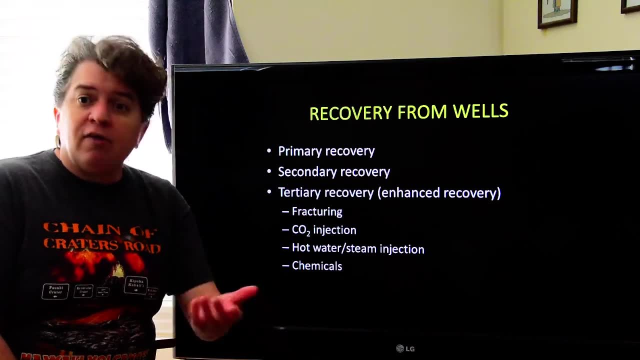 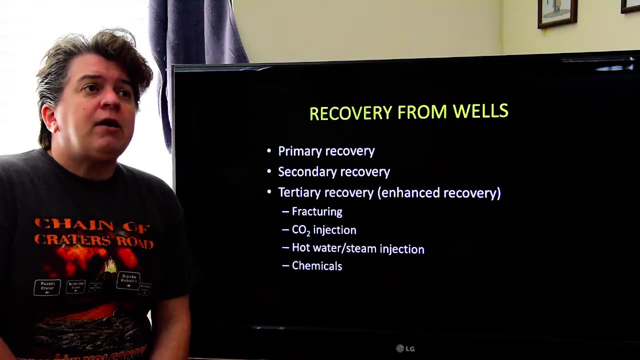 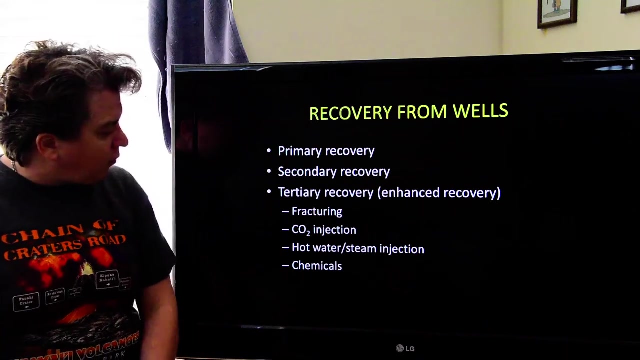 And in this case they might fracture the rocks, basically increase the permeability so more oil can flow, And I think everyone's heard of fracking. That's what we're talking about. There might be carbon dioxide injection, because carbon dioxide being a gas, can sometimes get into places that water doesn't and force out some extra oil. 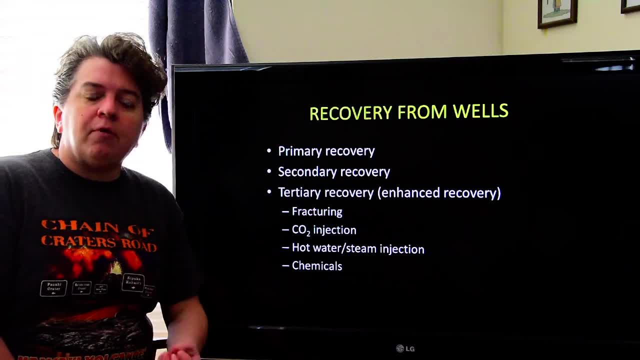 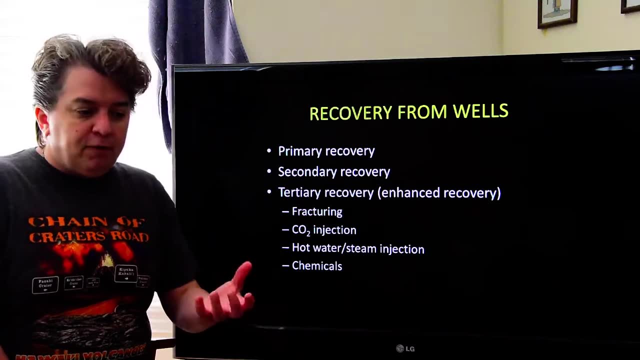 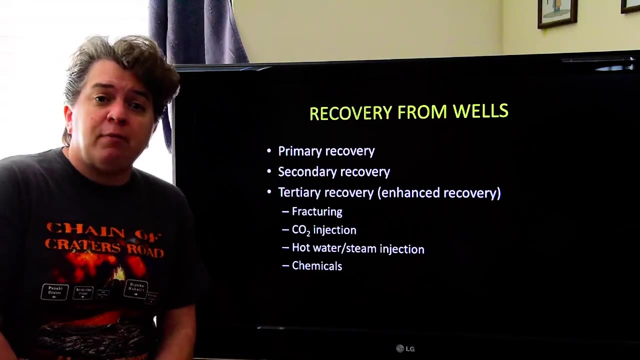 Sometimes they inject hot water or steam, Because what this does is they inject hot water And what it does is change the viscosity of the oil and make it flow better. And if it flows better, it flows easier into the well, And sometimes chemicals are used to accomplish the same thing. 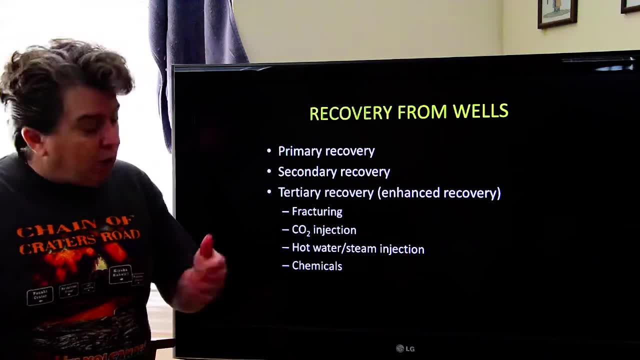 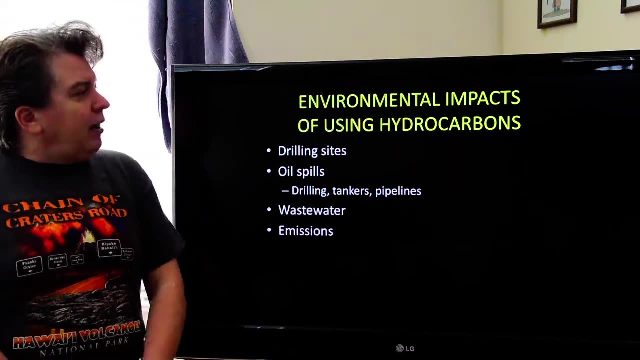 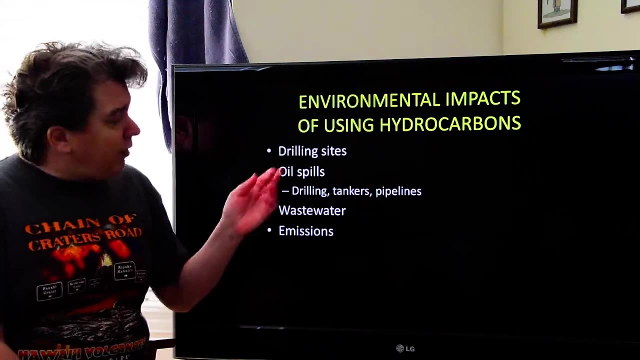 And so there are a number of different tactics that can be used once the easy ways of getting the oil are exhausted. Now, what are some of the environmental impacts of using hydrocarbons, using oil and natural gas? Well, you do have the drilling sites. 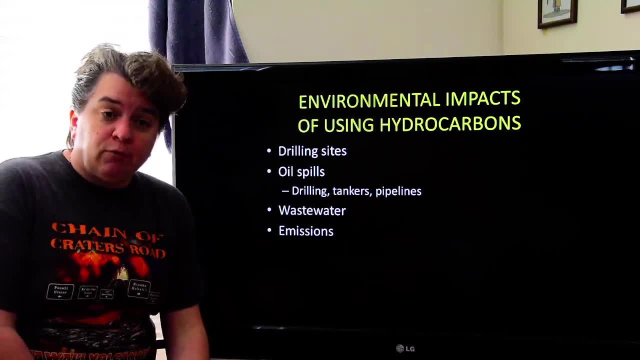 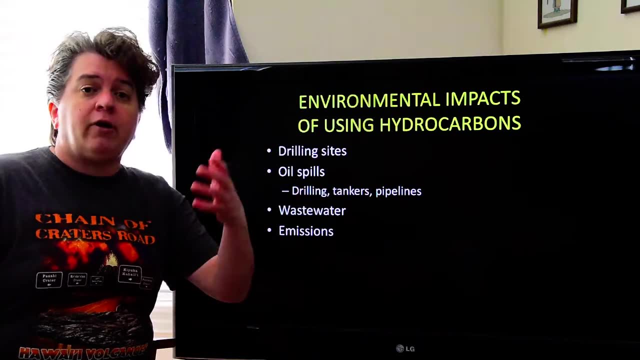 And so you're going to have to build roads to get to places where you want to drill for oil, And then you're going to have to clear an area of land where you can set up the rig and all of the equipment that's necessary for that. 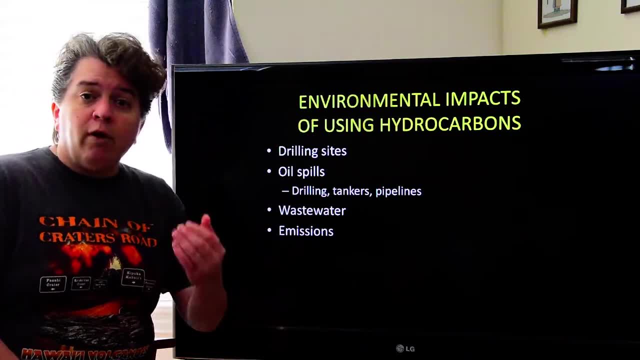 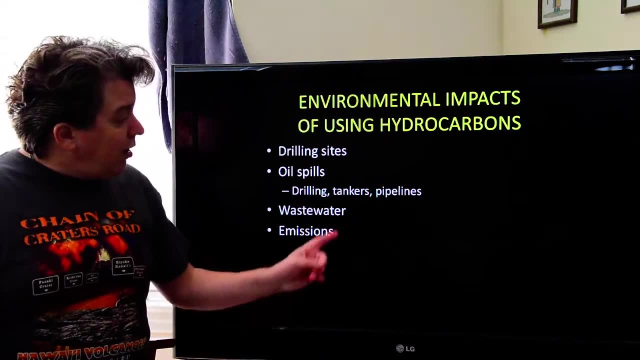 So you do have that. There's also, of course, oil spills, And these can come right from when you're drilling- Think the Deepwater Horizon thing- But also when tankers are transporting this oil, And then there's the oil spill. 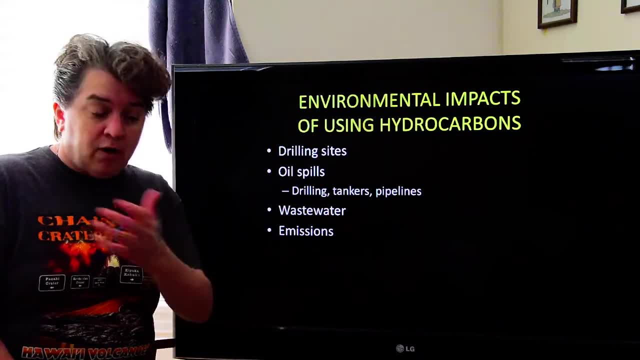 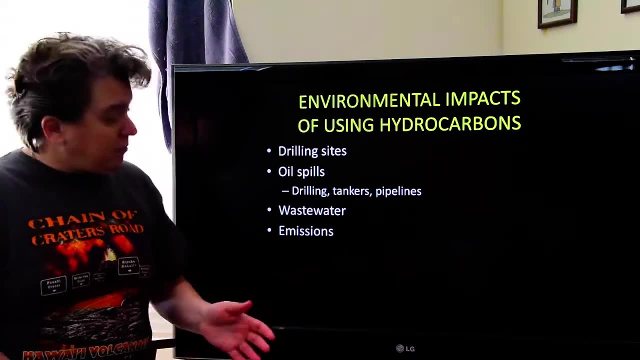 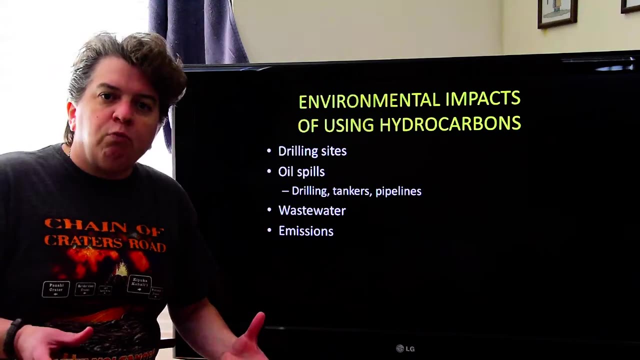 There's oil around, both on land and via super tankers out in the ocean. They can have spills, Pipelines can break, So you do have to think about those things. There's also the wastewater involved. I mentioned that there's always some of this water in these oil reservoirs. 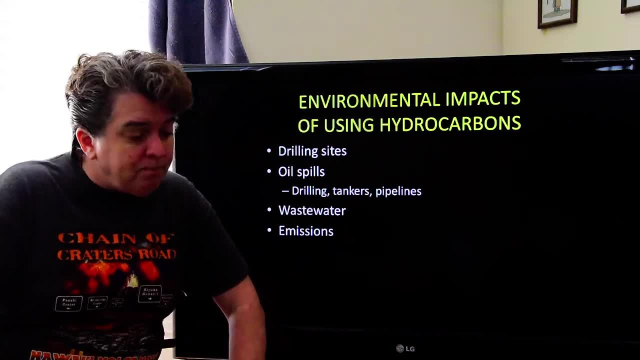 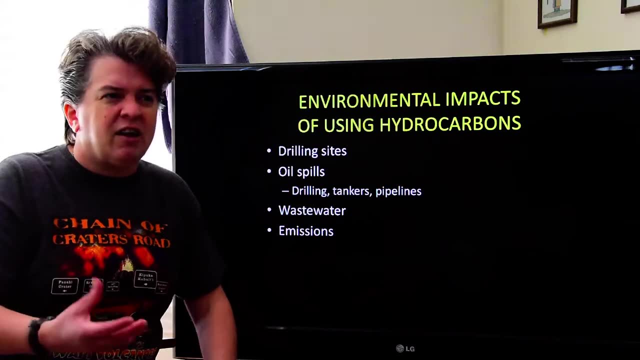 And when you're extracting the oil, you get some of that water as well, And this is not water you can just dump anywhere, Because, as I said, it's very salty And often also kind of sulfurous, And if you just dump this water out, that's going to be a pollutant.